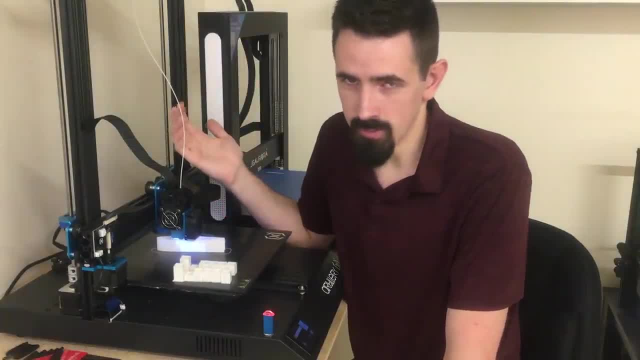 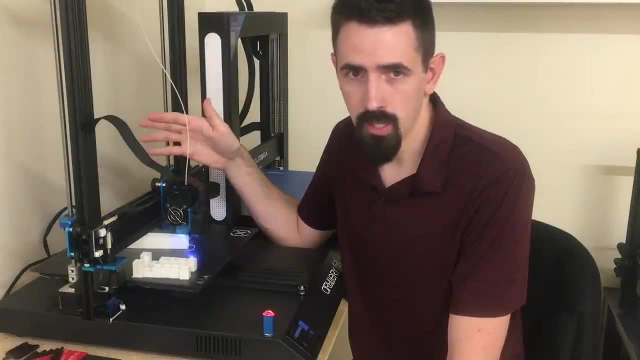 this stringing or anything like that and basically just have your retraction settings set off. I mean, it doesn't even, you don't even hardly need them on there at all, and it'll come out with a perfect quality piece every single time. and so if we take a closer look at this, you'll see that I have a part kind of rotated. 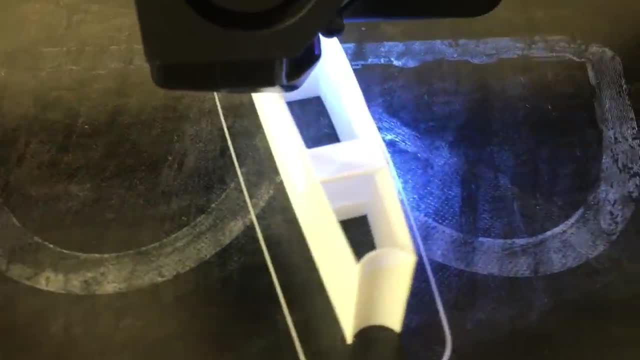 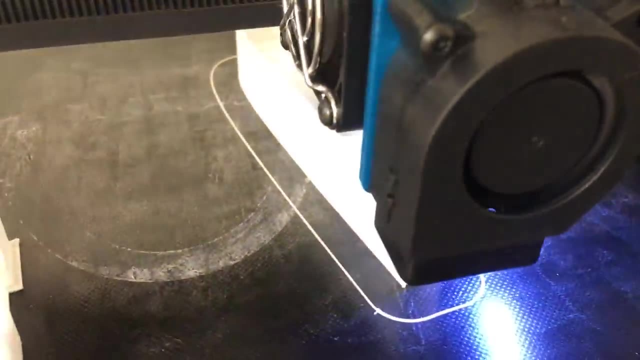 over. and then I have the z-seam set on the front axis right here and it's set to front and exposed. so it's set right here, so it goes all the way around and then it just gets to this edge and it moves up the next layer and keeps going. so you can see there that there's 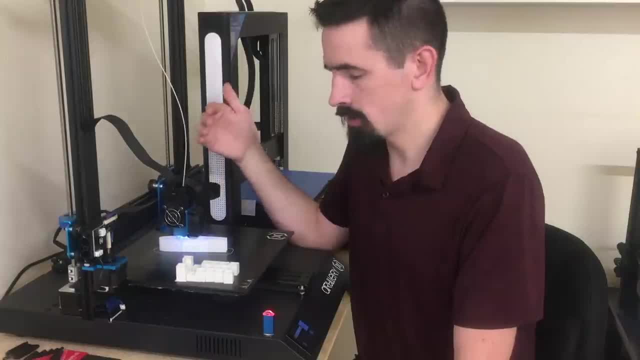 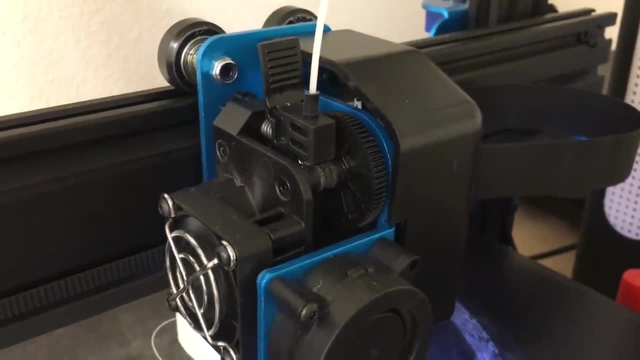 no stringing at all. it never retracts. that's why you know Eclipson particularly. it works really well with lightweight PLA because there's no retraction. and if you look a little closer at the drive motor on this printer you can see that it's just continually rotating. it never, you know. 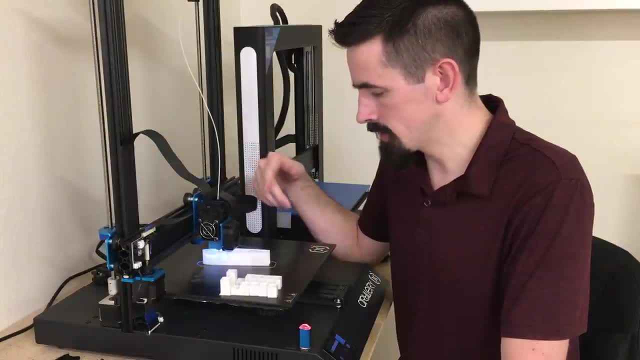 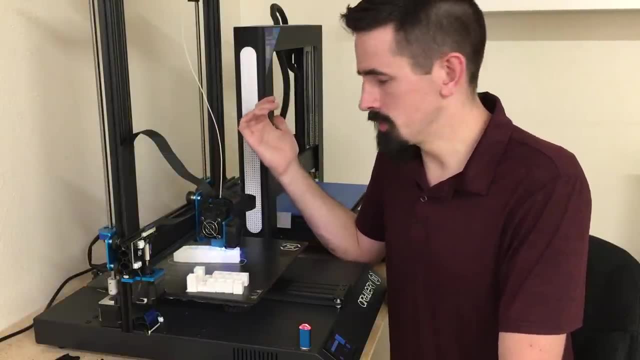 goes in Reverse, it just keeps, you know, pressing the material into the print. it never actually retracts, ever so this is with a direct drive printer, and I, you know, I use this to print all this stuff on my Bowden tube printers too, and it just like works perfectly. I mean, there's no you know inconsistency at all. it. 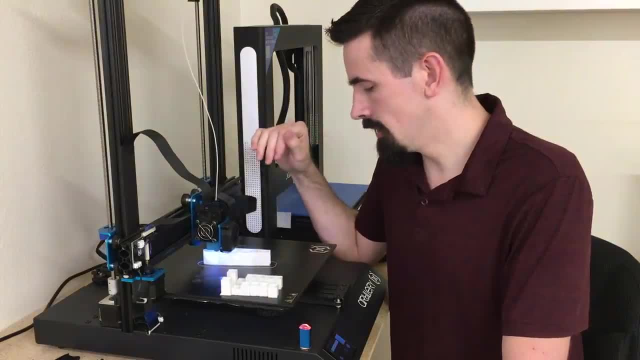 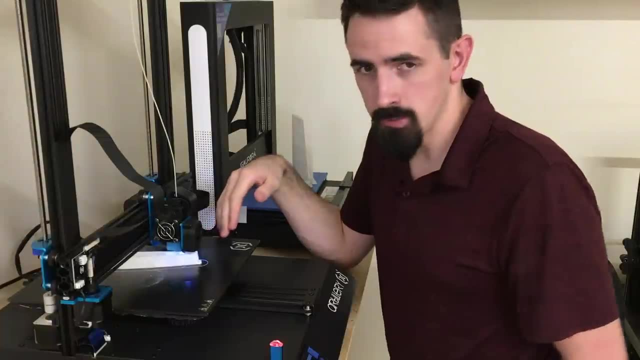 keeps the continuous pressure at the Bowden tube the whole time. you never have to worry about all this retraction kind of settings. okay, now I've got a 3D lab print wing from the Cessna 152 that I did and you can see the. 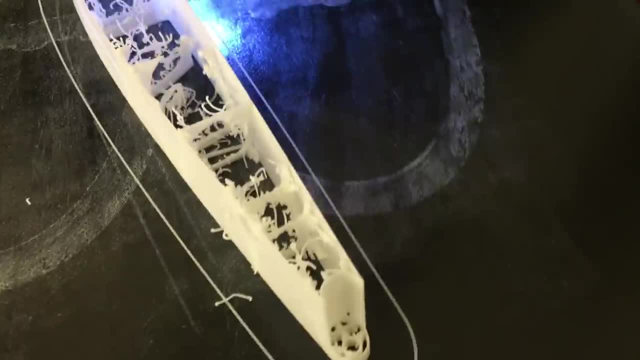 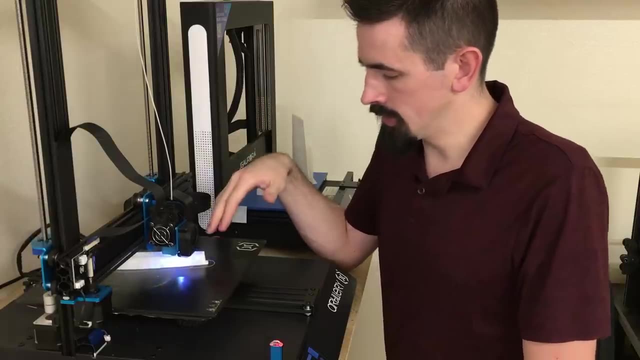 between the Eclipson wing and this wing. see the inside of the wing. it's got stringing all inside. here you can see the driving motor how it's retracting, priming, retracting, priming. the stringing inside the wing isn't completely bad I. 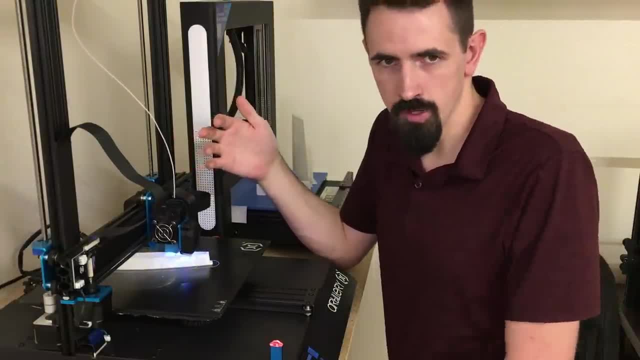 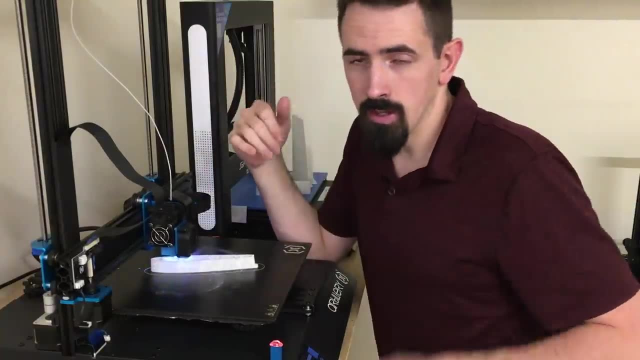 mean you can still print it. it doesn't add a ton of weight to have that stringing in there. it'll work just fine. but inside the wing it's gonna look pretty bad. and then you hold it up to the light you can definitely see like the stringing on the inside of the wing, but where it comes, you know, problem too. 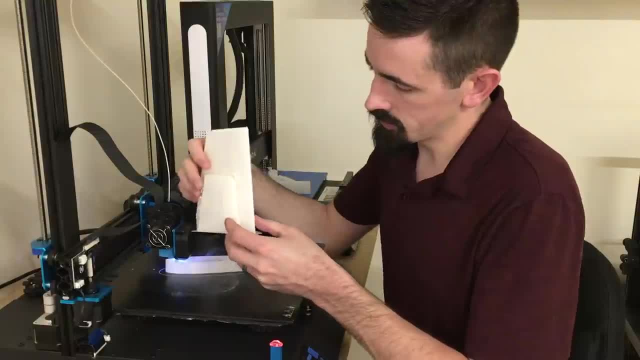 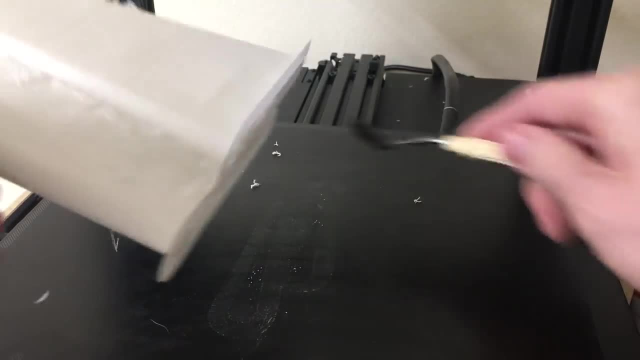 is if you're gonna print off like two parts like this. you know these are two parts printed together and you can see that. you know this is the result. you've got stringing all between the parts. they're gonna clean all this up now. there's not a way to eliminate that with. 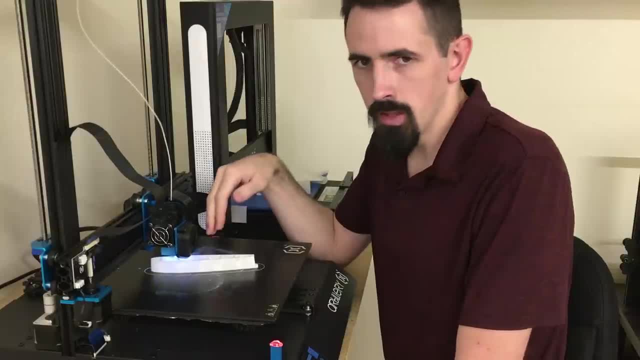 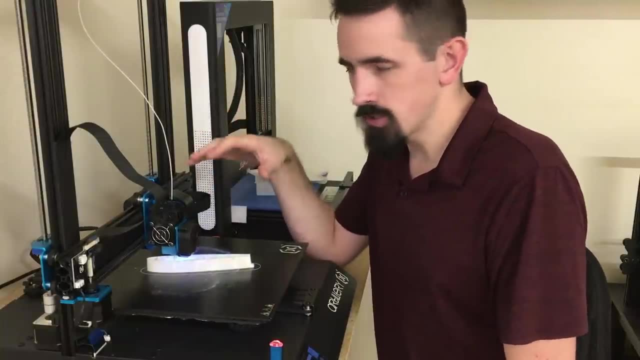 the wings. you know the extruder usually stays within the wing is fine. but when you're printing a few swatch part and like you have a hollow center and where the battery tray and all kind of stuff is at, well, you're gonna get stringing all in that area. so you got to clean all that out and it's kind of a pain. so 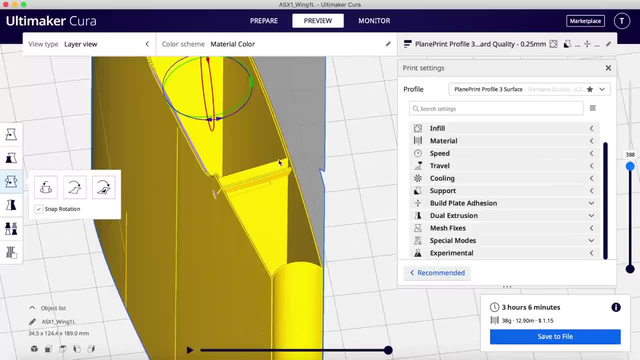 let's take a little bit closer. look in Kira. so you're just gonna take a little bit closer. look in Kira. so you're going to take a little bit closer look in Kira. so, with the eclipsin part, you can see i have the travel line set on and there's no blue lines. 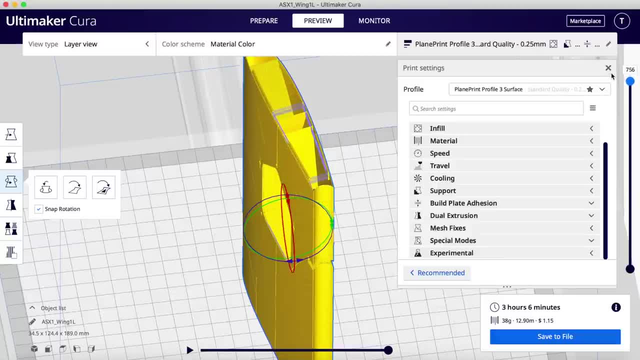 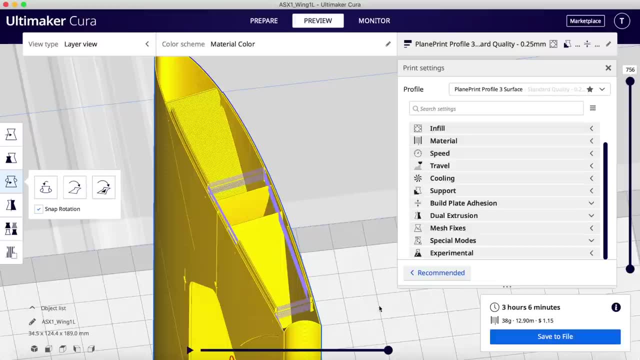 anywhere on this part, except for on the very, very top where you print the tabs to assemble the wings together. there are some travel lines there, so that's the only travel lines or attraction and priming settings on the eclipsin wings on the very, very last few layers now you can see for the 3d. 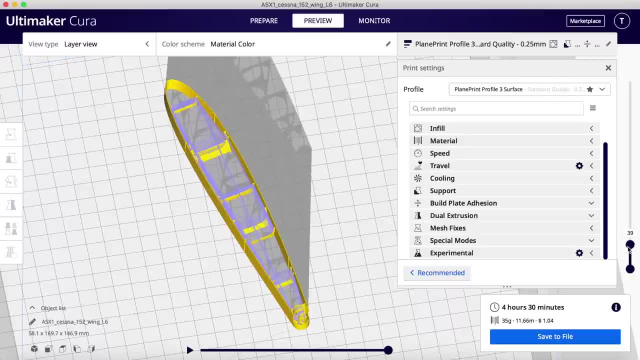 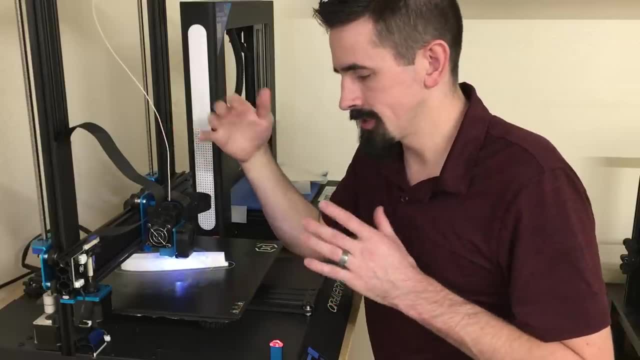 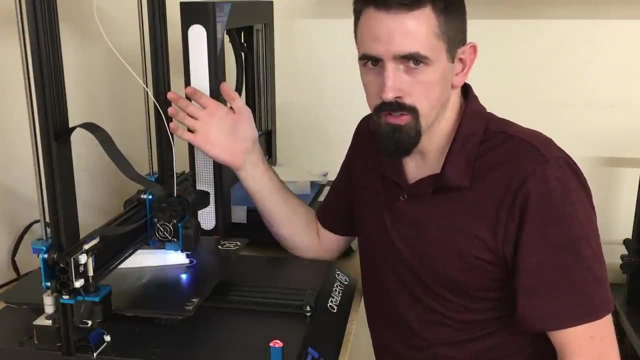 lab print wing. the entire center of the wing is covered in blue lines. that's because it's traveling all over on the inside of there. to sum it all up, basically, as long as you're printing an eclipsin plane, your pla and your lightweight pla are going to print identical. there's going to be no. 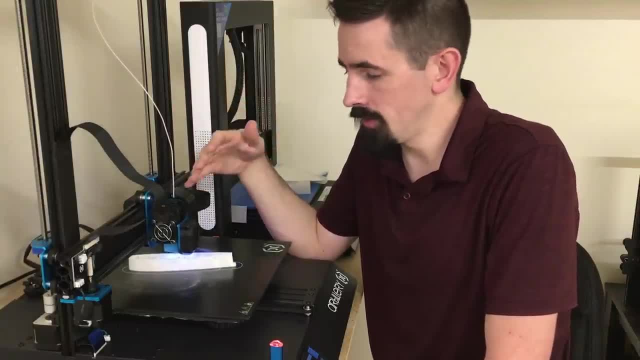 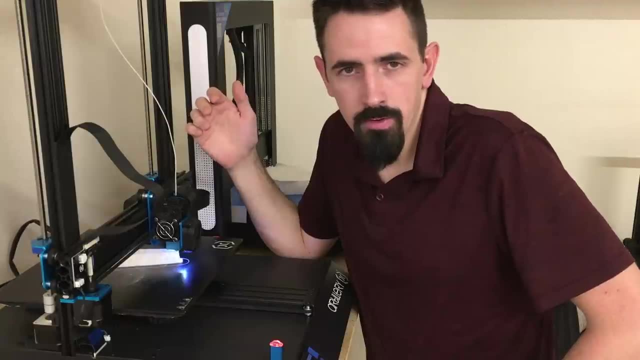 difference between difficulty as far as printing lightweight pla or printing pla. now, when it comes to other planes, when you're going to print, if you're going to say, like i'm going to print a 3d lab, print 152 out that i already did, like. 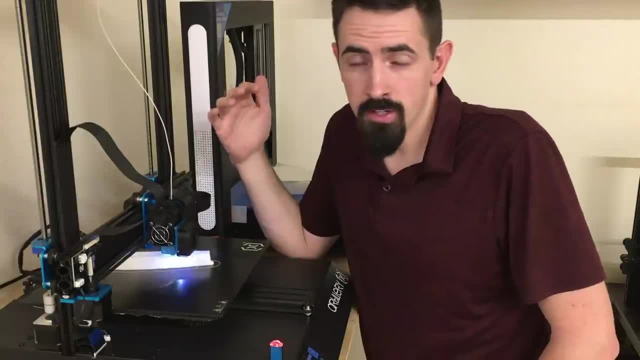 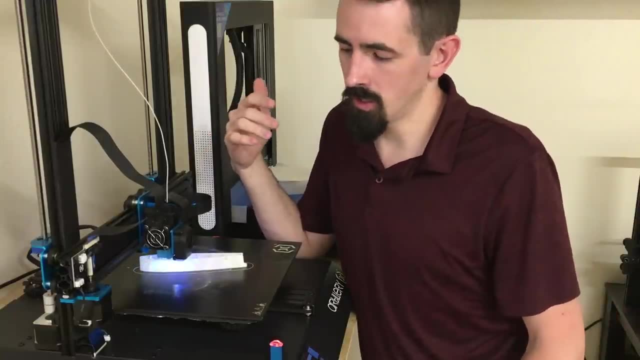 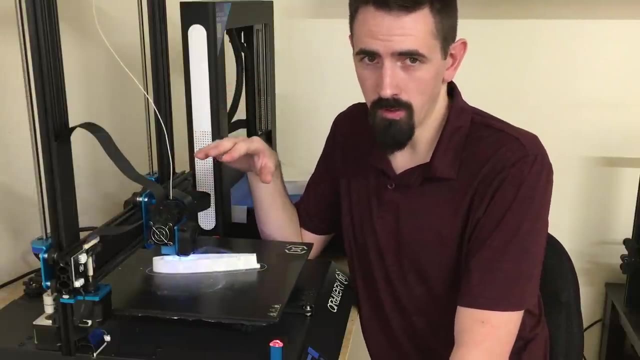 uh, you know you're kind of getting into uncharted territory at that point. you know you're kind of tests, you know in testing phase there, because this hasn't been tested see. so eclipsin actually is the only company out there that has designed all of their airplanes to work with lightweight pla. so 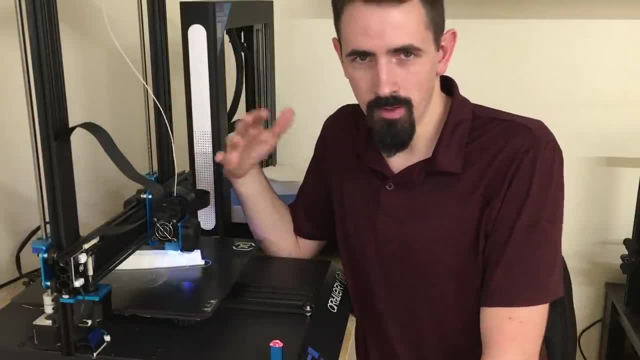 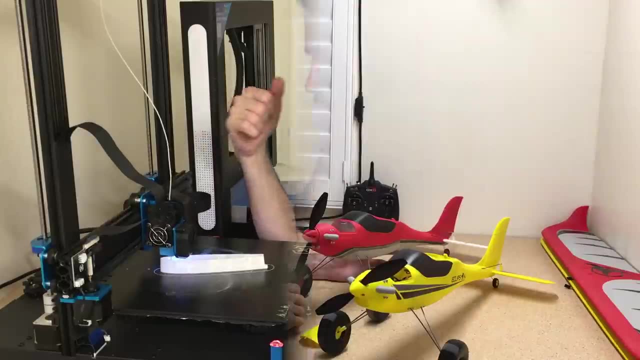 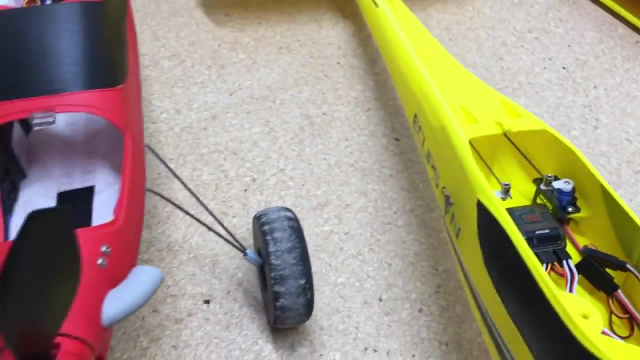 the designer basically has to design the plane to be available to work with lightweight pla and if they haven't, then you know, like i said, you're in kind of charter territory- may or may not work. so, taking a little closer look at the model c's, they're completely identical. all the pieces are the same. i have all the same receivers. 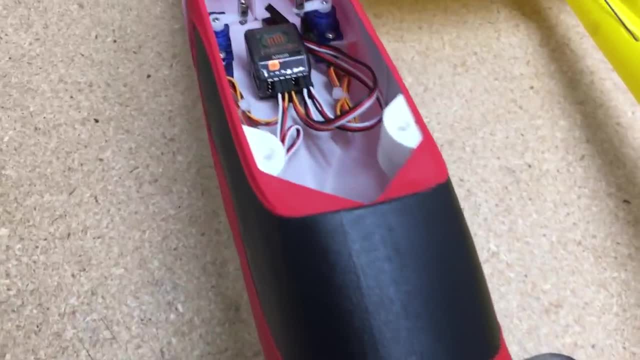 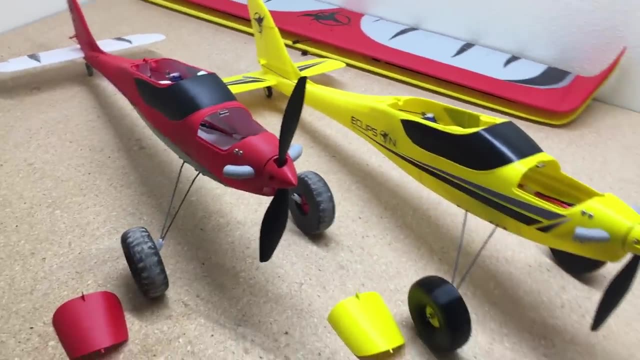 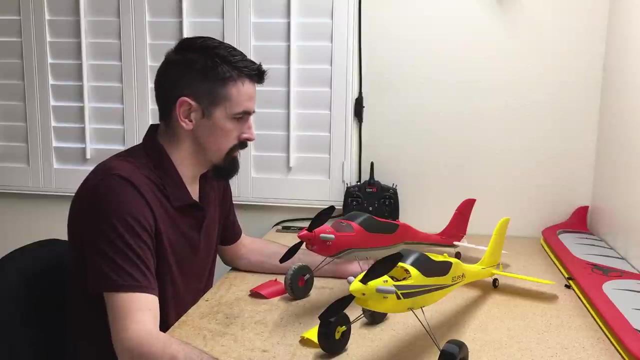 motors, servos, everything set up the same. the uh lightweight pla version is just painted red. that's one disadvantage to lightweight pla is only comes in white or black and the you know pla get that any color you want. um, so another disadvantage of it is the cost. so you only get uh lightweight pla from colorfab and another one so depending on 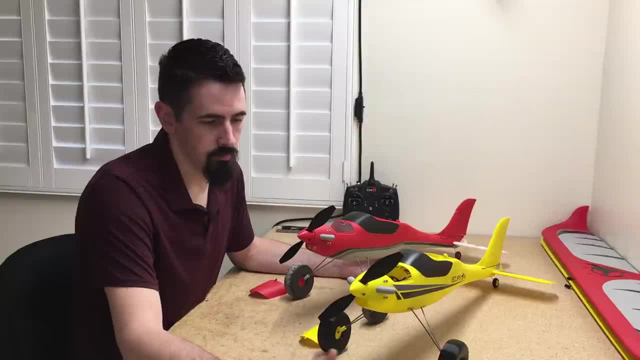 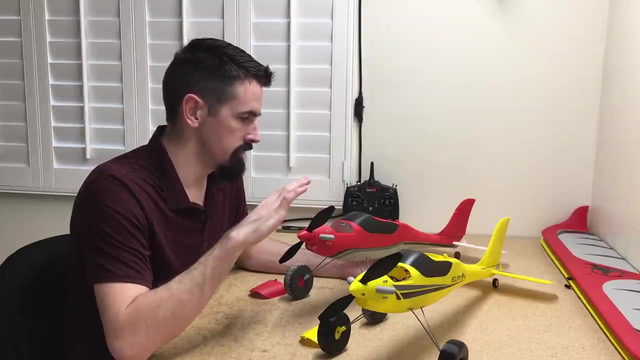 where you're going to ship it to. that can cost some money and the product itself is like twice as much as regular pla. but the difference is too you have to think about is you're printing pla at 100 flow rates and you're printing lightweight pla 53 flow rate, so you're actually going to be able. 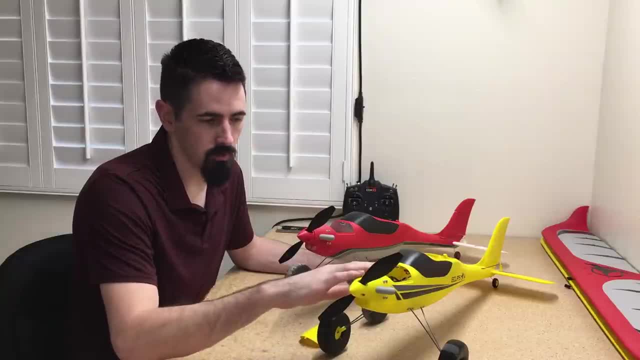 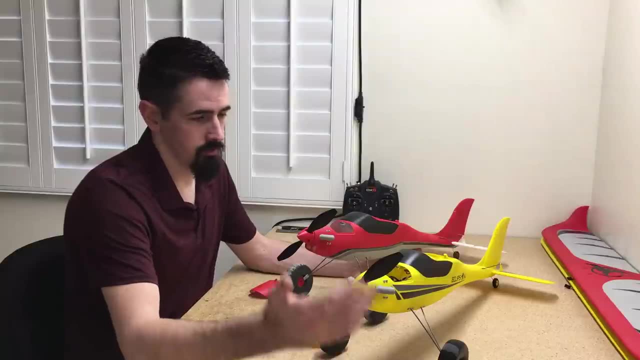 to print more airplanes out of the lightweight pla version than the pla version. something with eclipson planes. it is nice the continuous printing that it does. it doesn't do any retraction, the parts so like in this whole plane, uh, with the wing and everything. it's like 48 hours of continuous. 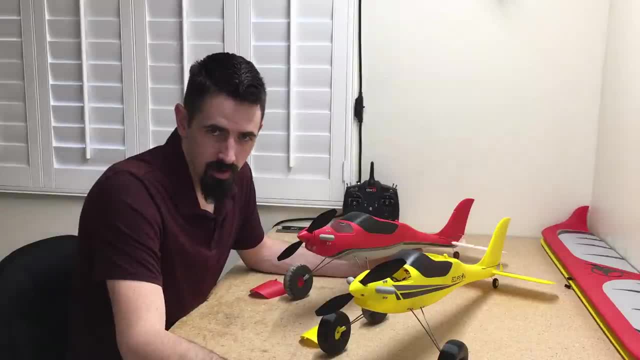 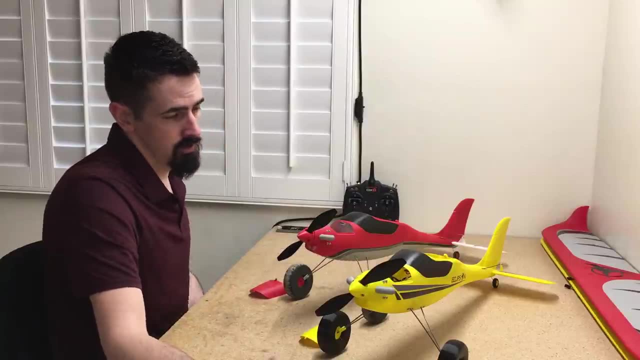 printing, whereas you know anything else is like hundreds of hours of printing. i mean you could print just one section of wing is like 12 hours or something like that with other other companies. so, uh, with that minimum- you know movement of the extruder, it saves a ton of time. 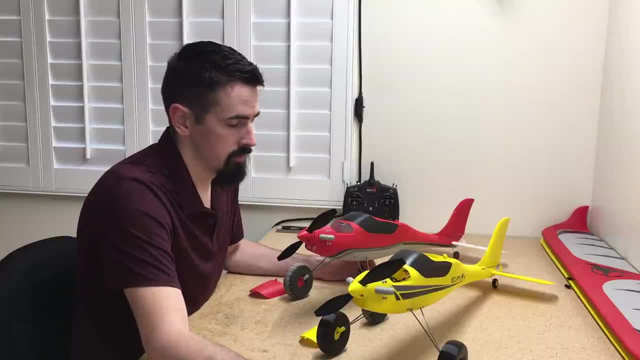 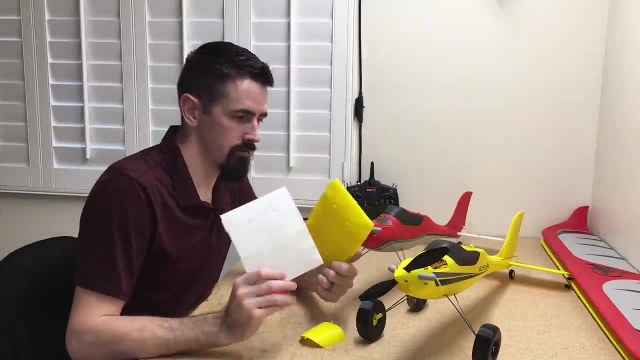 and just way easier to print. so that's something to keep in mind also. okay, so the next thing that we're going to do is a little bit of a strength test. so i have two parts: i have a pla and a lightweight pla part, so i don't have any fancy tools or anything. i 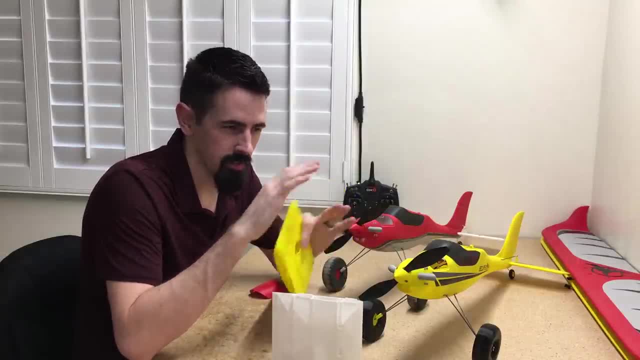 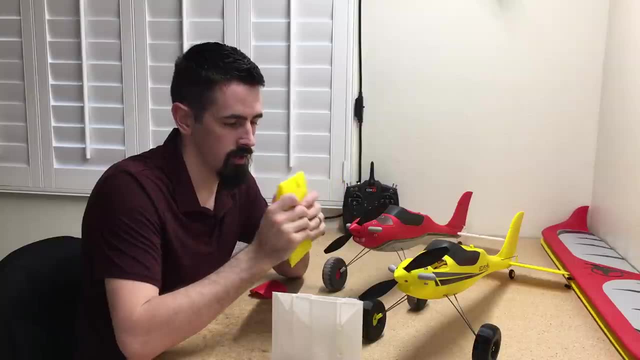 can really like test the strength of this with or put it on some tests and, like you know, give you an exact number for like what the strength is. but i'm just going to try to break these, i'm going to try to break this skin with my finger and i'm going to try to break this in half. uh, 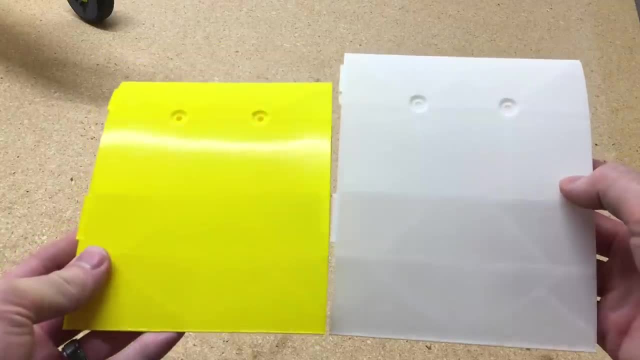 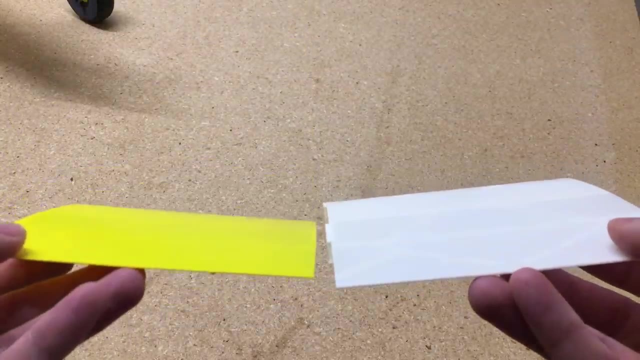 the other thing is like the finish. if you look at the finish on this, this is nice, smooth, glossy finish. the lightweight pla is kind of like a fuzzy kind of finish to it, not like perfectly smooth, it's not like glossy, it's like a flat white kind of. 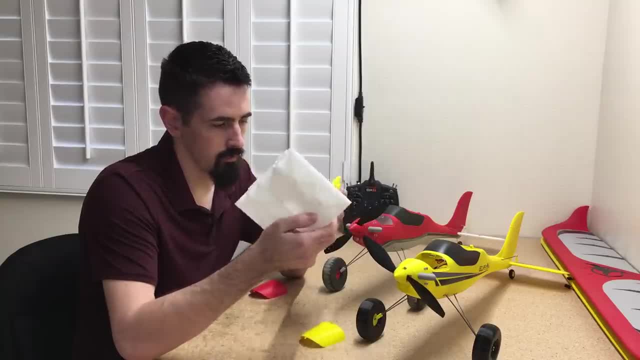 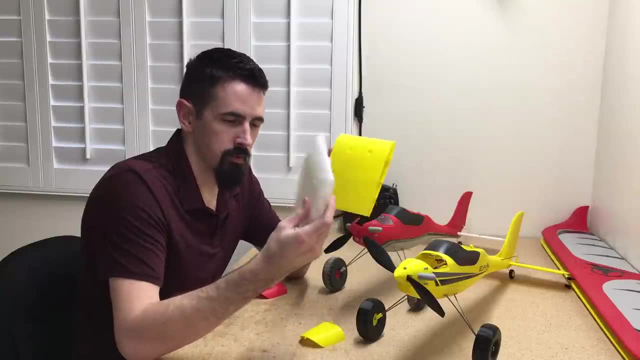 so that's a little bit of the thing, is just the look of it. so we're going to try to break these. you know, definitely you can. you can just feel the surface of this is a lot, uh, softer than this, but something with the strength of this, uh, that you do need to keep in mind. 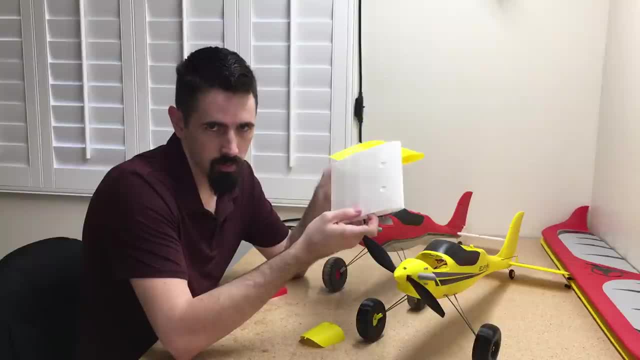 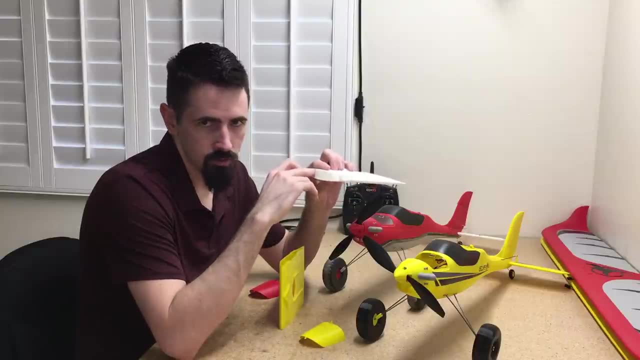 is eclipson has designed all the airplanes to be printed with lightweight pla and so their wing design. if you look inside the wing, uh, the structure inside is completely solid. there's no slots or holes inside the rib sections in the fuse, in the wing or the fuselage. 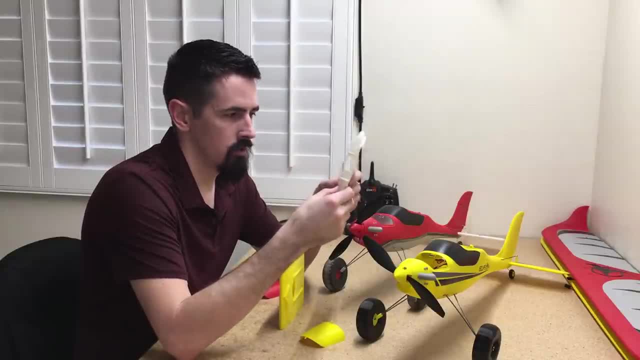 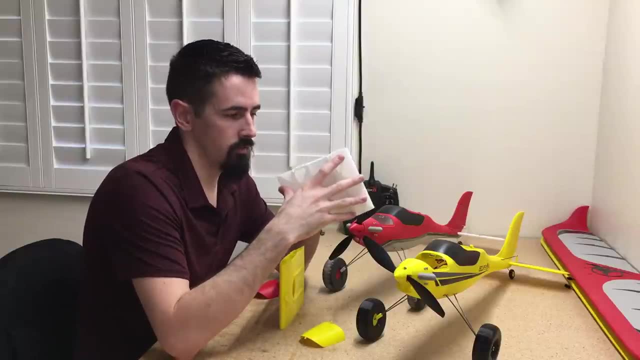 so that's designed to work with lightweight pla, because they know that the p, the lightweight pla, is not as strong, so they actually, you know, reinforce the material more in a lightweight pla airplane, but in in the end of it all, it all saves weight anyways, because the lightweight pla 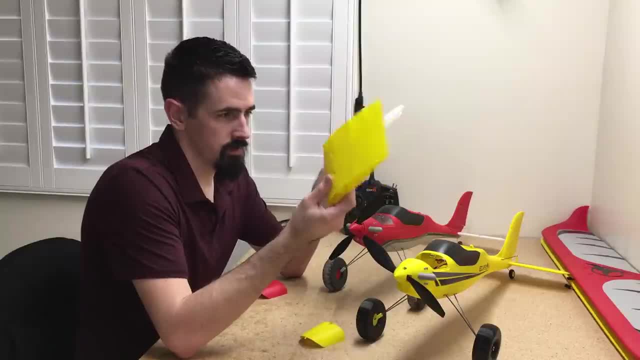 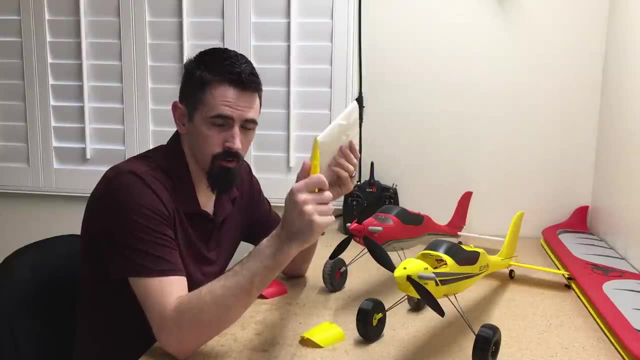 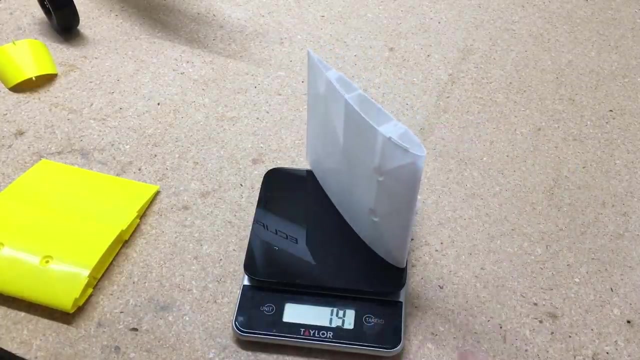 is so light, so um, but then if you print the same part out of the pla, it still is fully filled on the inside of the wing and it's very strong, but it's heavy also. so first we'll just we'll weigh these. so for the lightweight pla we have 19 grams, and for the pla, 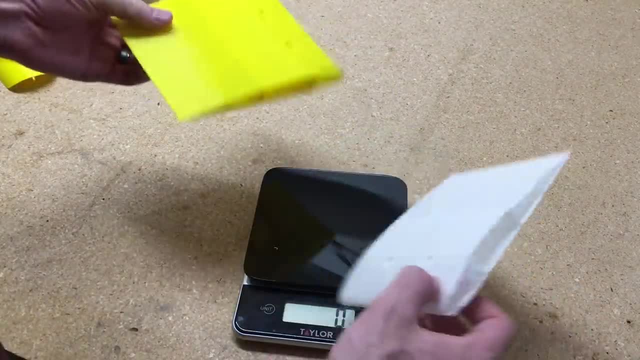 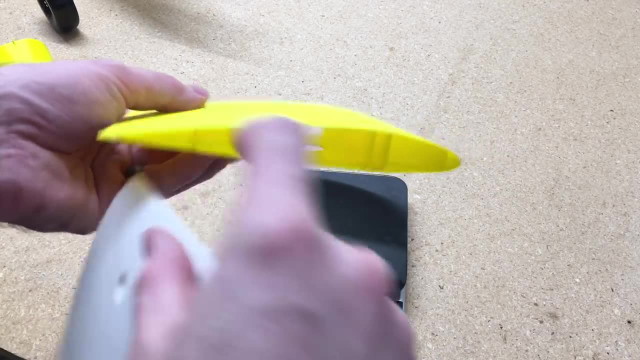 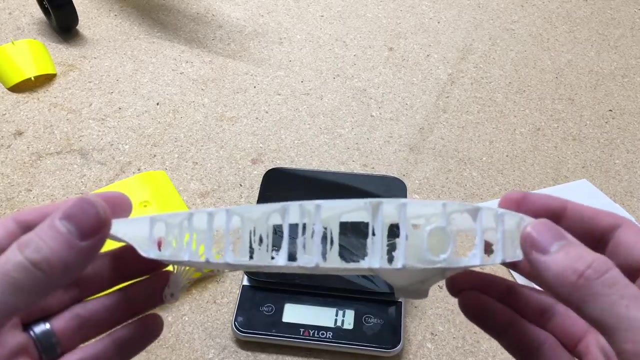 we have 43 grams. so that's the same part. and then you can see the inside. you know how there's. there is a hole here for the servos and then here there's no like slots here. and same with the lightweight pla version. so if you look at a competitor wing, this is like a 3d lab print. you know inside of a wing and it's. 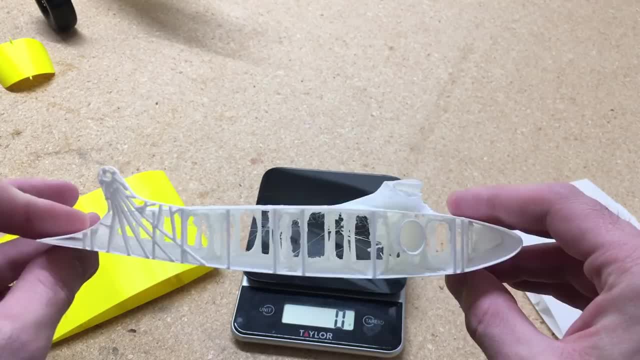 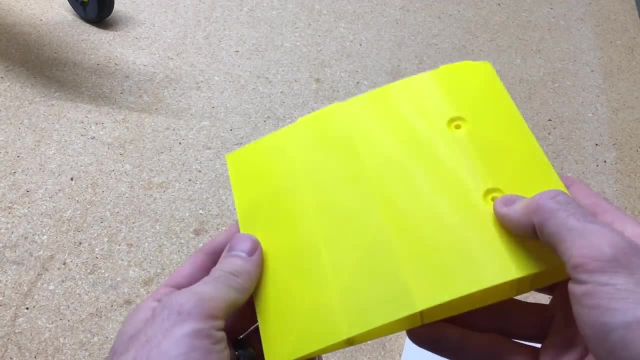 just completely open now. this is a really bad print. this is a pretty old piece that i have, but you can see just the difference in structure on the inside of the wing. so what i'm going to try to do here is actually break the skin of this. so let's try to do it. on the lightweight pla version. 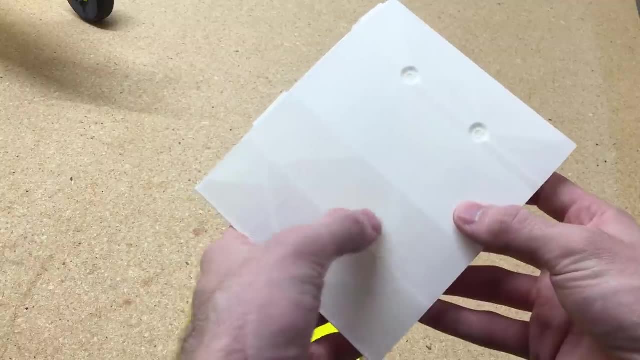 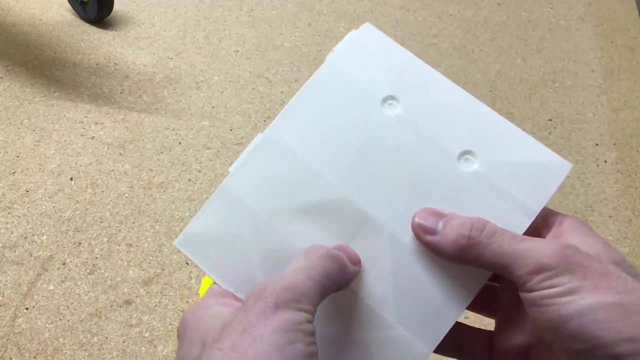 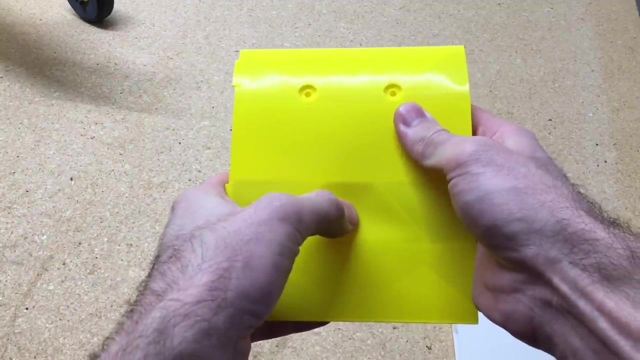 first, so you can see, kind of, here's a rib section, kind of between. here i'm going to try to actually break this with my finger. so just without much, without much pressure there, i've just cracked it. now let's try it with the pla version. so pushing pretty way harder than 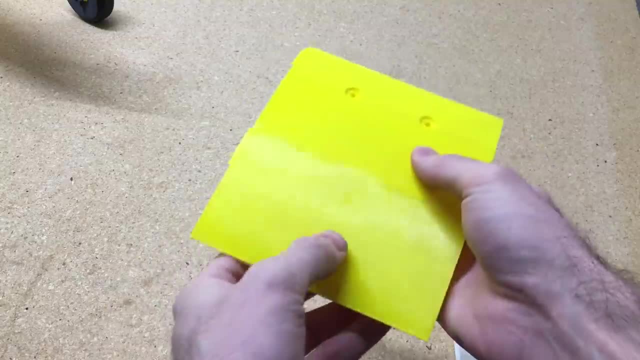 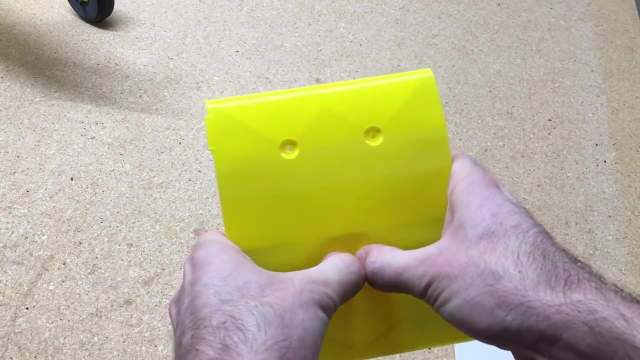 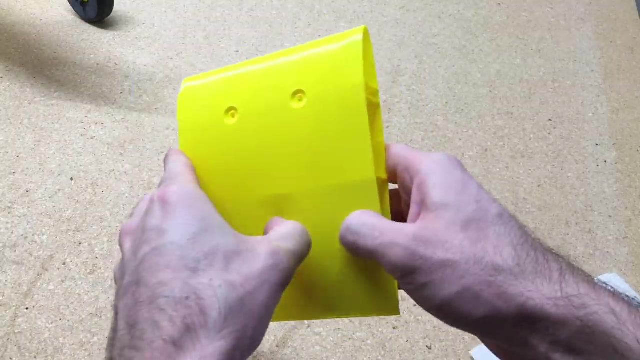 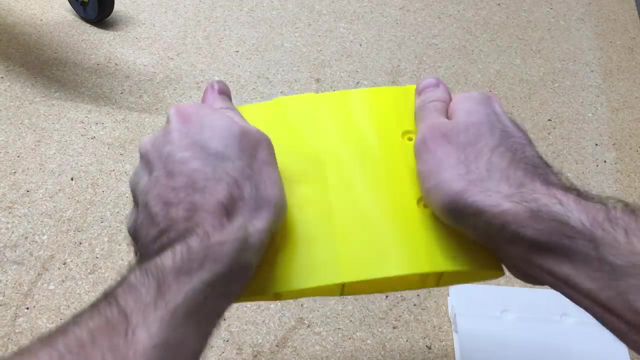 the other one and it's like bending here, i can't actually get it to to break. wow, that skin is strong, that's just, it's very strong. there we go. i got it to break, there we go. so, yeah, it's, it's way stronger, uh, than the lightweight pla and then turning it like this way, twisting it. 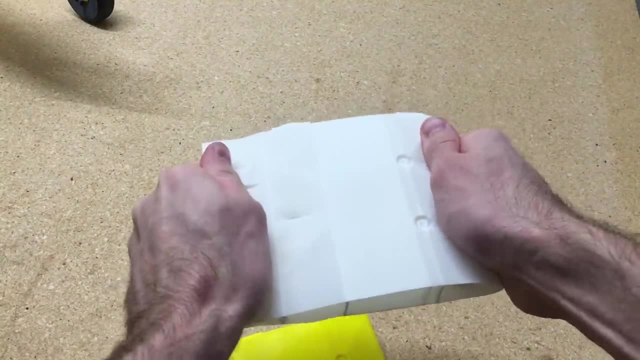 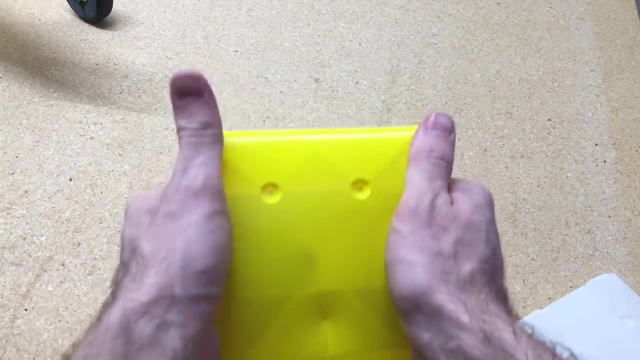 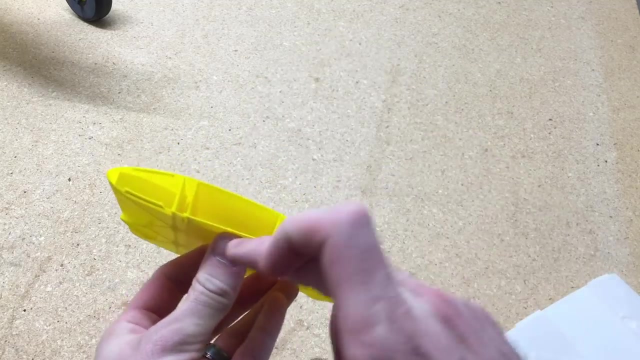 you know it's very strong, you know, versus like this one, definitely you can twist that and break it. now let's, um, let's try to actually break it in half. so let me see this: so right, here is actually two layers thick here. so, like, this is two layers thick here. this is kind of works. 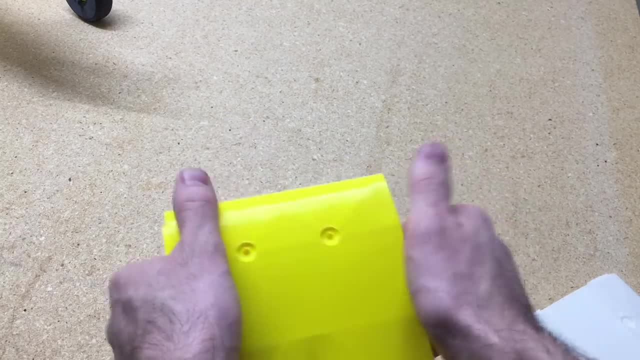 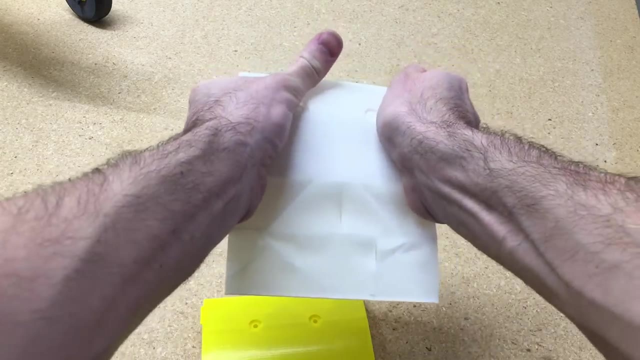 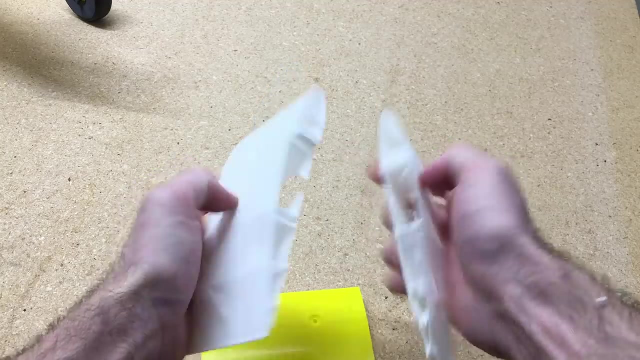 as like a spar in there, how strong that is. so i'm going to try to just break it this way. let me try it with the lightweight version first. yeah, there we go. so, yeah, it broke. uh, right there at the seam. uh, it's pretty strong. let's try to do it with the pla version now. 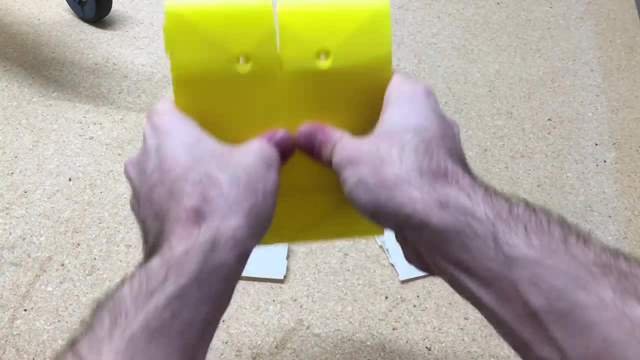 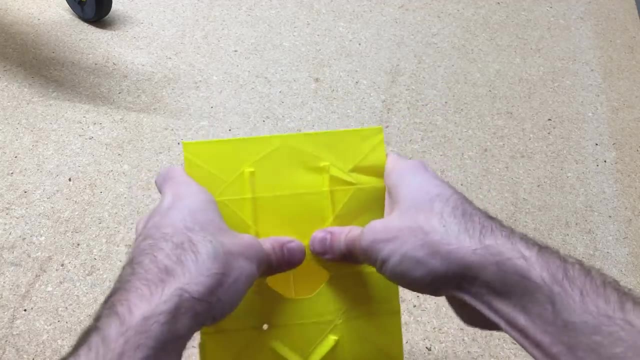 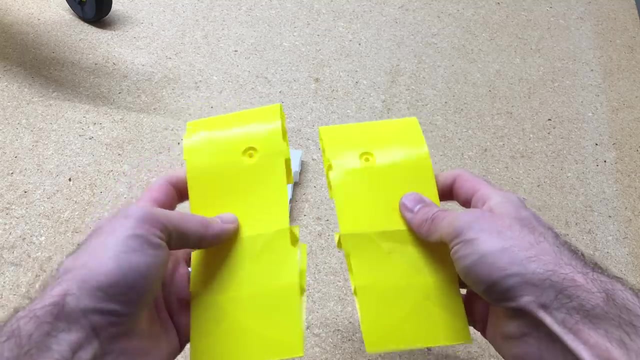 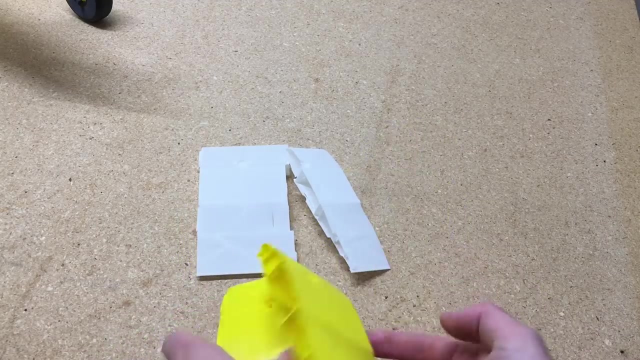 there we go now we got that to break. so that's definitely a lot stronger, you know, than the lightweight pla. um, but you know that was, you know you don't usually do that with your regular wing, okay, so definitely the pla wins the strength test for sure. 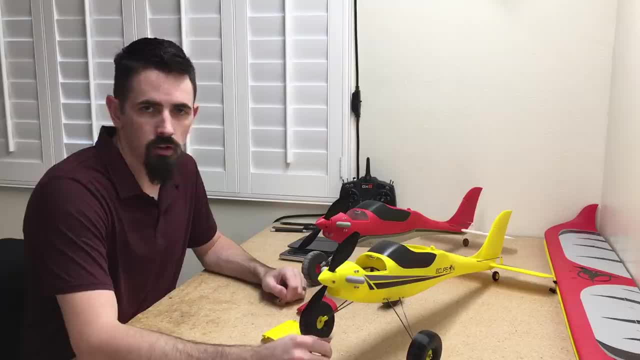 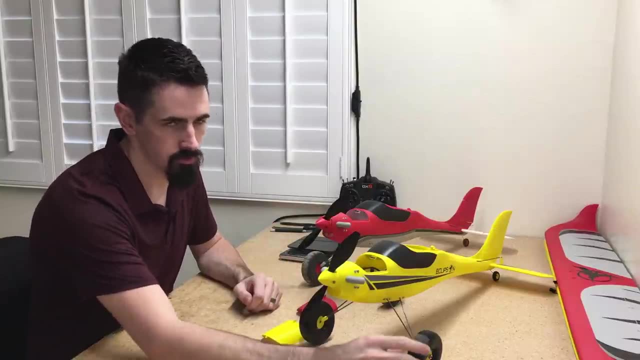 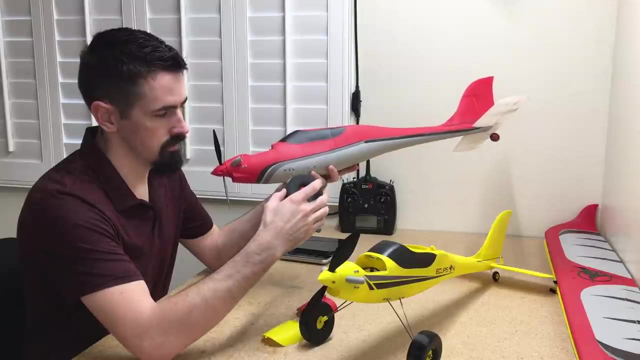 uh, lightweight pla is definitely not as strong. okay, the other difference between these two airplanes are the tires. so, on the tires, for the pla version i used just regular tpu and for the lightweight pla i used a very sure tpu by colorfab. so this is a also another. 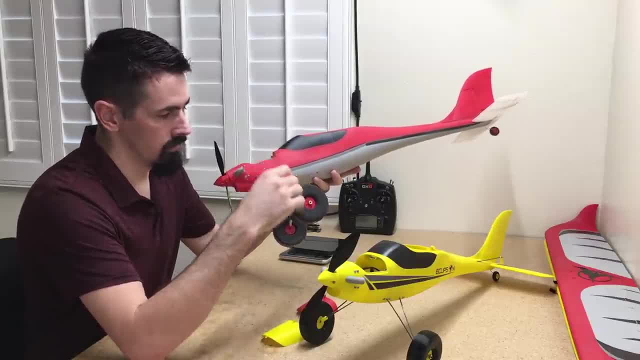 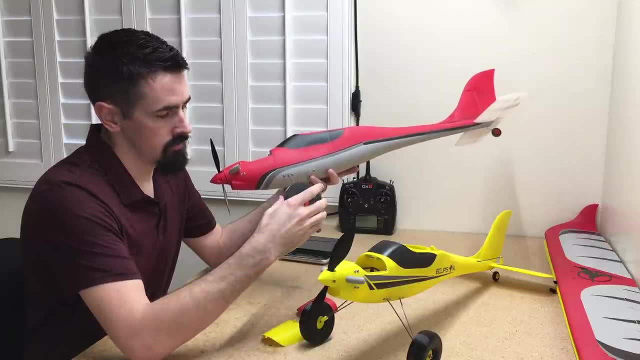 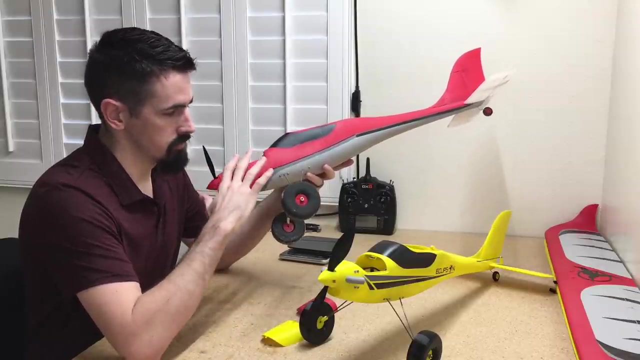 material that works just the same as the lightweight pla, where it has a foaming reaction and makes the part way more lightweight than regular tpu. the other thing that's nice about it is it's a lot squishier, so it has a lot more like shock absorption on the landing. so for like this. 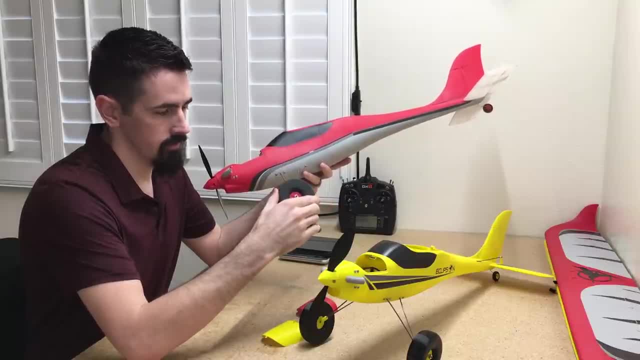 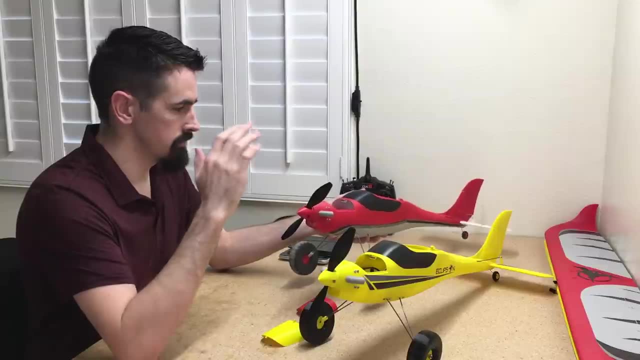 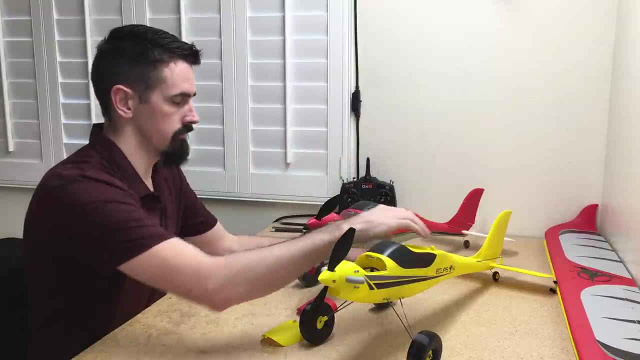 bush plane where the tires are kind of oversized. uh, you know, this bearish or tpu definitely helps with cutting down the total flying weight for the airplane. uh, now, as far as assembling goes for the two airplanes, uh, they're pretty much identical other than a few parts. so as far as 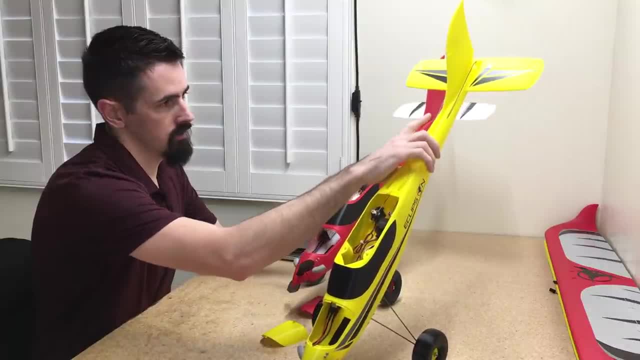 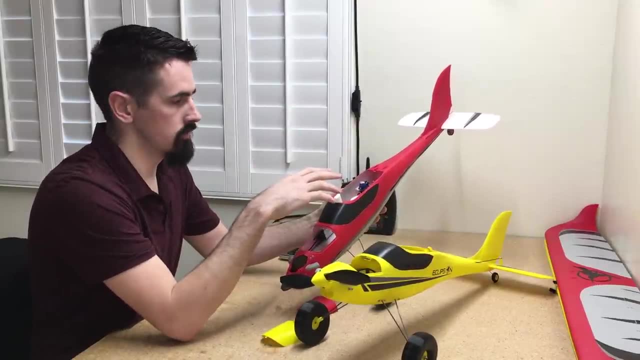 like for these two airplanes, uh, in the tail section. uh, for this airplane, uh, there's no carbon rods uh inside of the rear part of the fuselage, but in the lightweight pla version, eclipson recommends to have, you know, carbon rods for this tail portion here. so that's one. 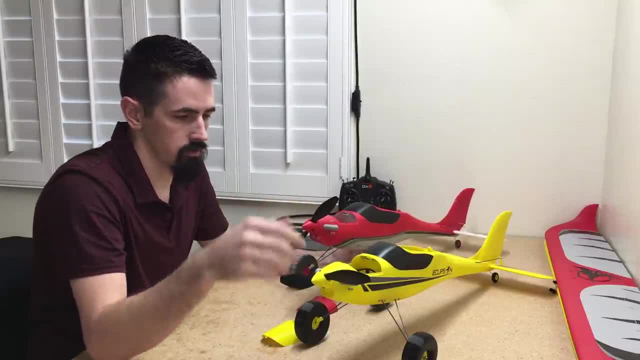 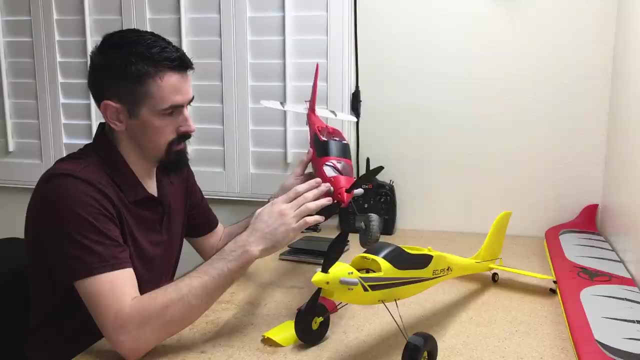 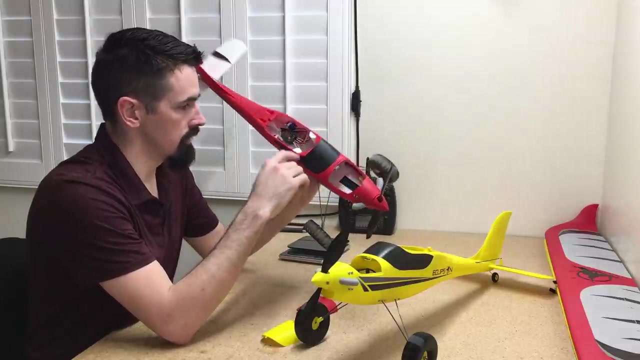 difference between the two models. and then there are a few things that are printed out of regular pla, like for the lightweight pla version, like we'll start, like the spinner here, the accent pieces for the exhaust pipes, the parts for the landing gear, here are regular pla. these 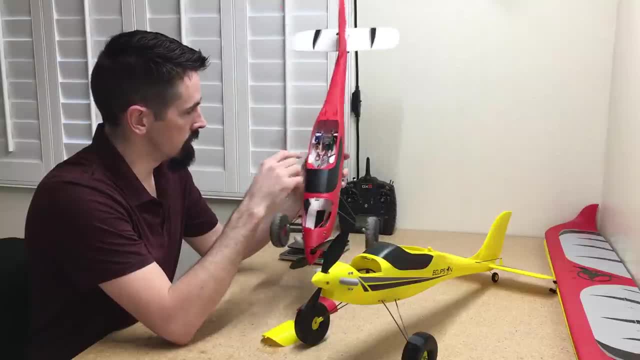 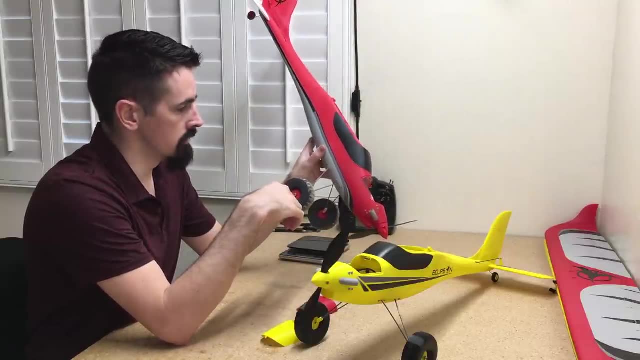 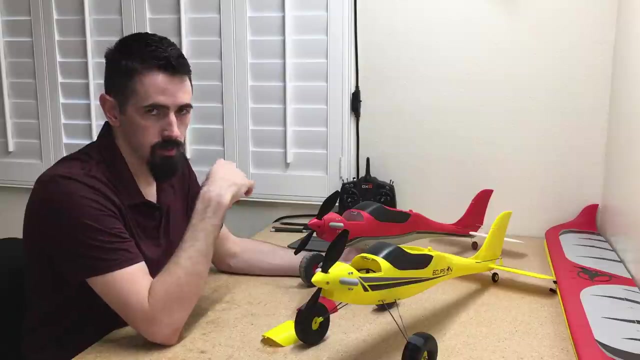 wing support pieces are pla, the servo mounts for the wing and for the fuselage and then, like the rims for the tires are regular pla. so there are some, some, a few parts that are just regular pla within the lightweight pla model to keep it strong. so you know parts that are you know or like the. 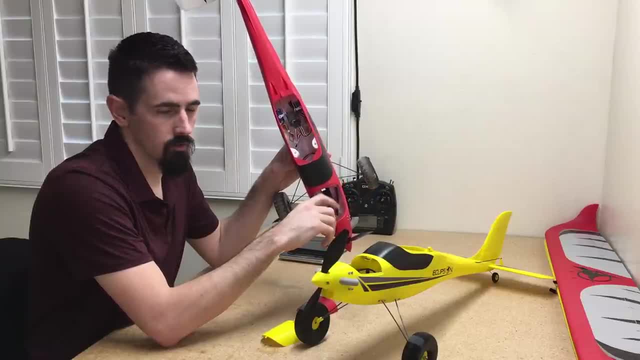 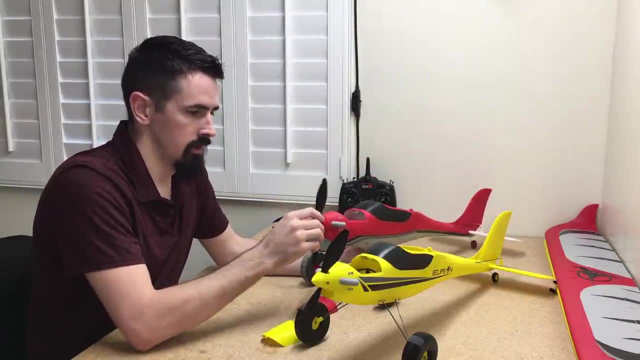 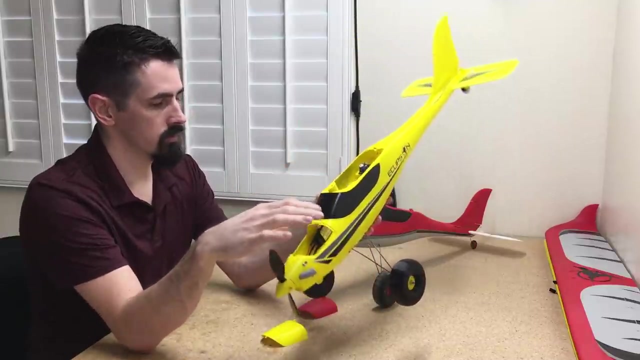 you know the engine mount is printed out of petg or abs for the temperature resistance. so a few differences like that. whereas the pla model you can just print like all the parts out of pla, i mean the whole fuselage, print out. these are all printed out pla, all the wing. you know everything's. 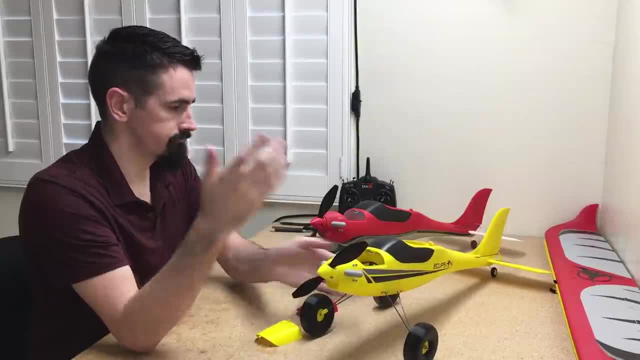 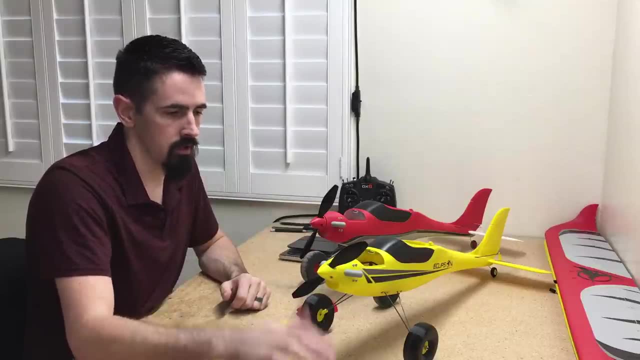 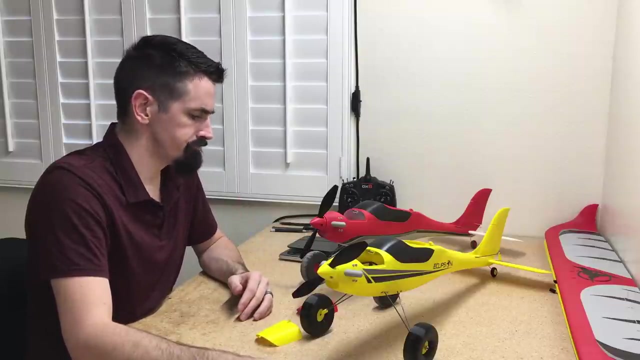 printed out in pla, um. so that's one difference there. so the assembly process is is equally easy. for lightweight pla or pla, the printing process is the same, like i said for each one, as long as you're doing the eclipson airplanes, um. so let's- uh, let's, throw the wings on them. 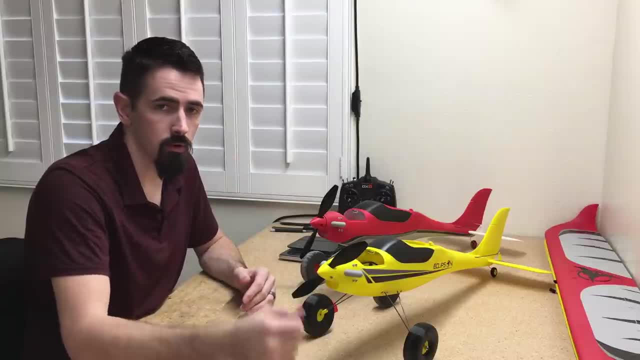 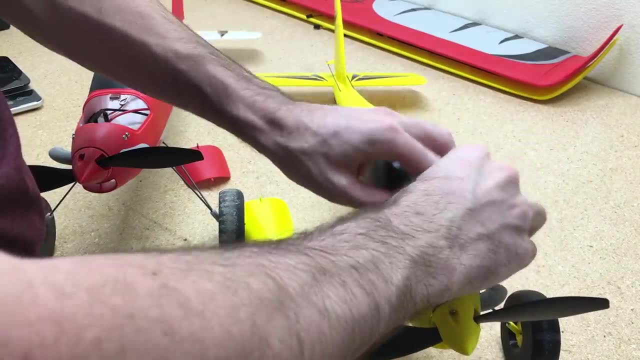 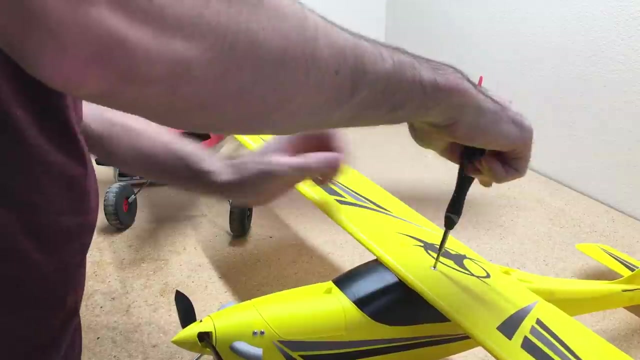 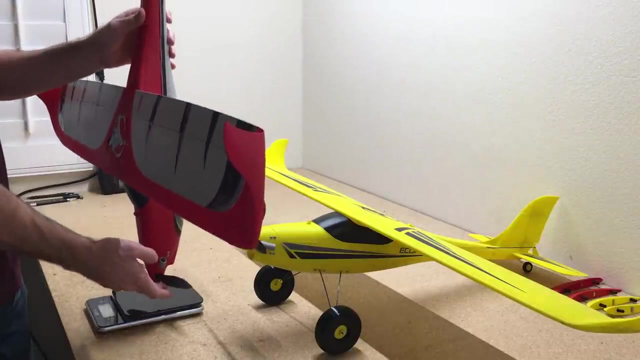 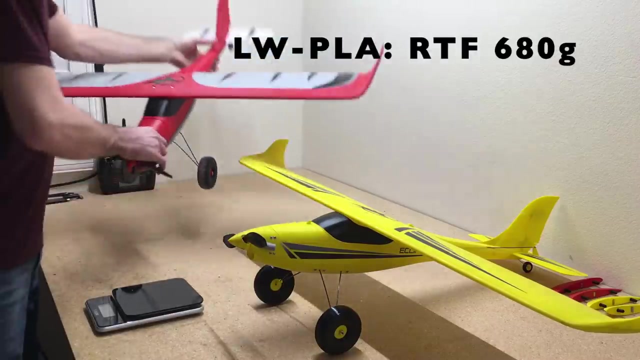 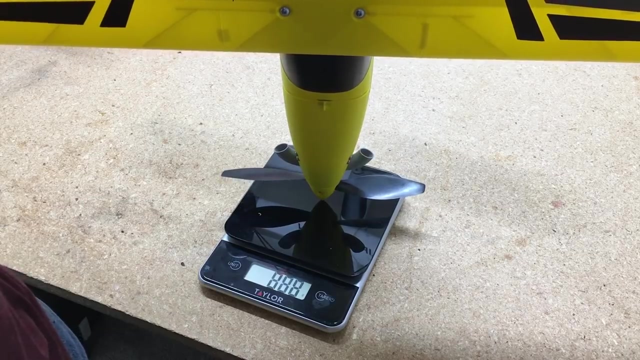 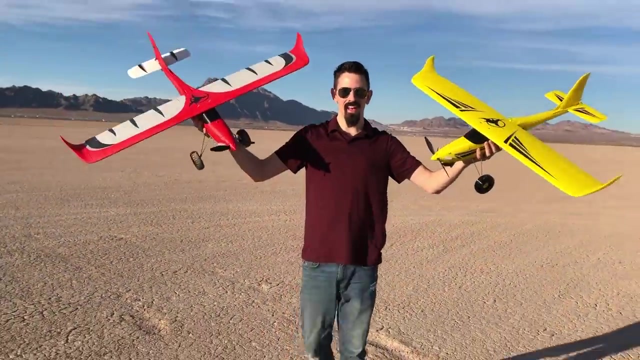 put the batteries in there and let's get it ready to fly weight, and then we're going to be taking these out to the desert and trying to fly them. okay, so about 680 grams for the lightweight pla version. okay, so there we go. we have both the planes completed- pla and lightweight pla, this one. 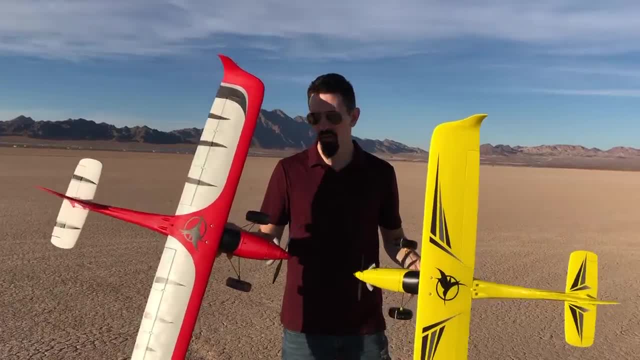 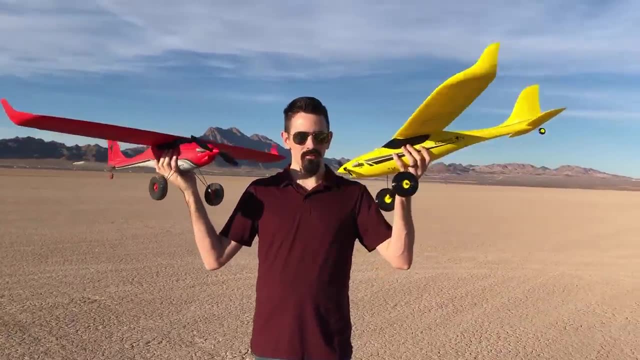 is 210 grams more than this lightweight pla airplane. so we're going to take them out here and see how they fly, and we're going to test these out and see which one flies better and see what you can get flying slower. so let's- uh, we're going to try this lightweight pla plane first. 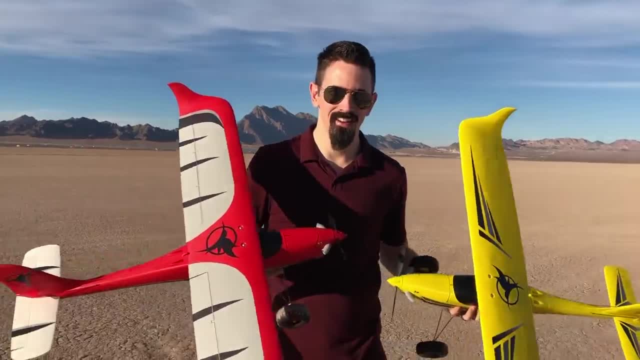 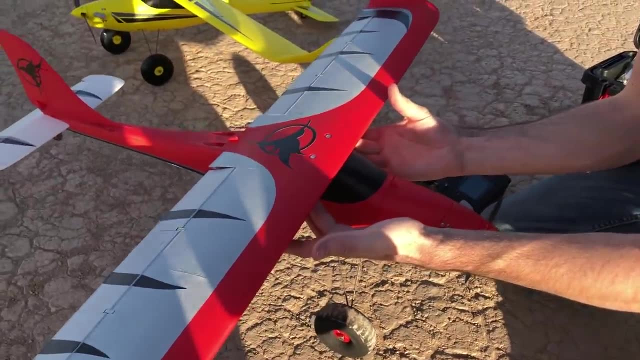 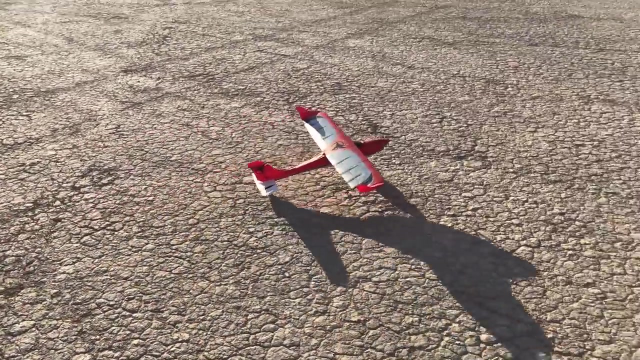 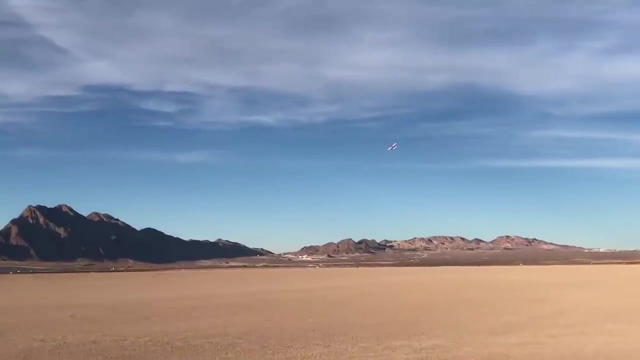 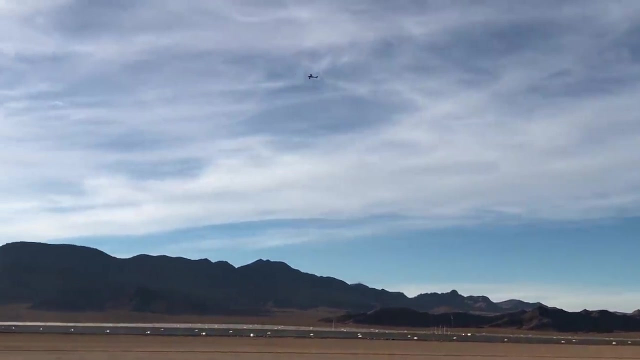 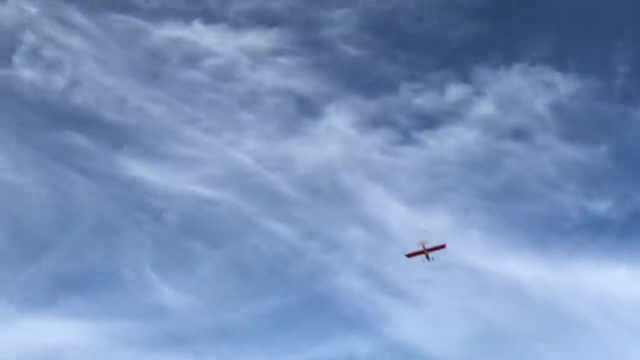 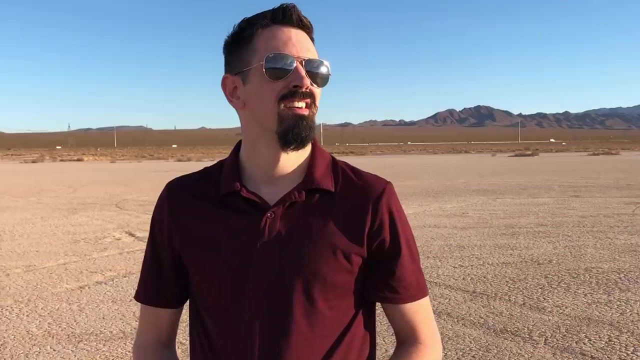 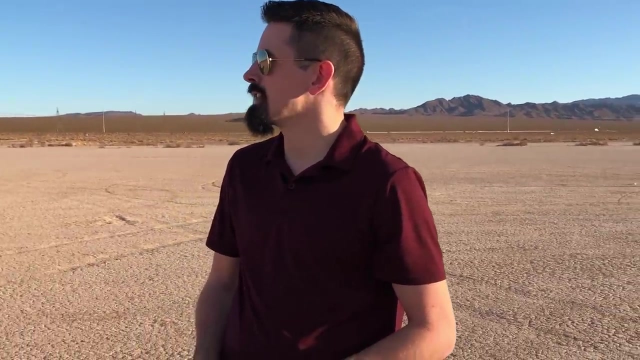 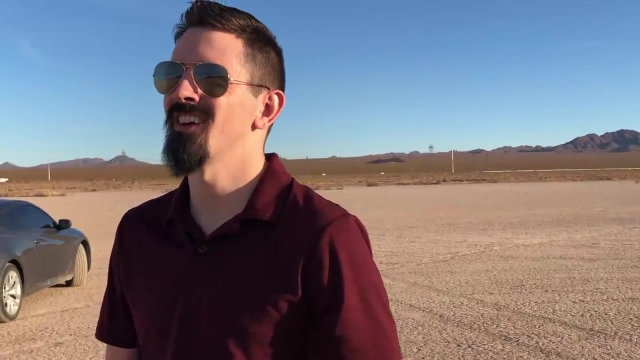 and then we'll go with the pla airplane. so let's go ahead and get these ready. okay, we have it flying on the lightweight pla airplane. it's flying really well. put in some flaps then you can get it flying really slow. Just really good flying a little plane. So let's get this one on the ground. 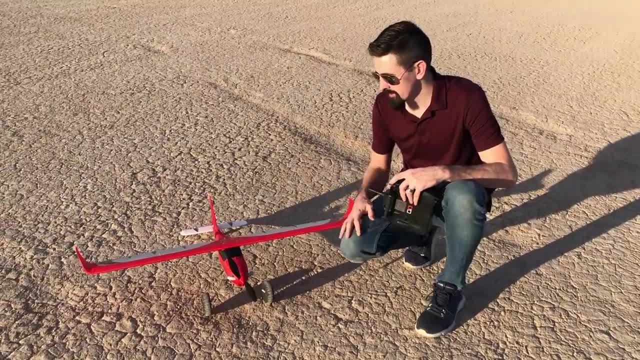 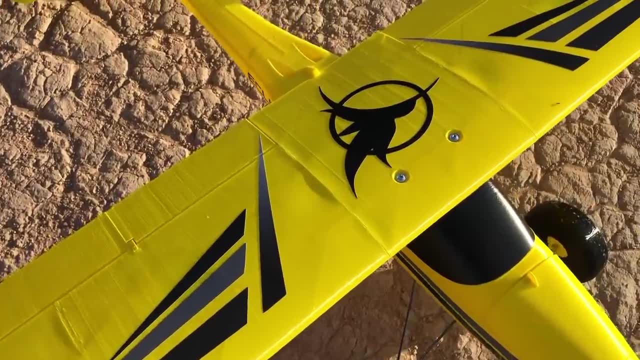 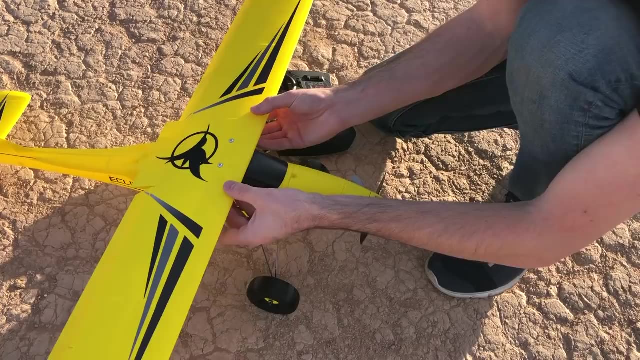 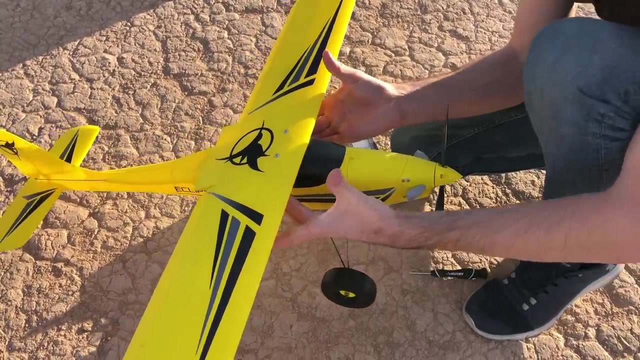 Okay, so that went really well with the lightweight PLA version. the plane flies really well. it flies nice and slow. So let's get the PLA version set up and we'll try that one out. Okay, so that's a little bit of problem. CG is a little bit aft. 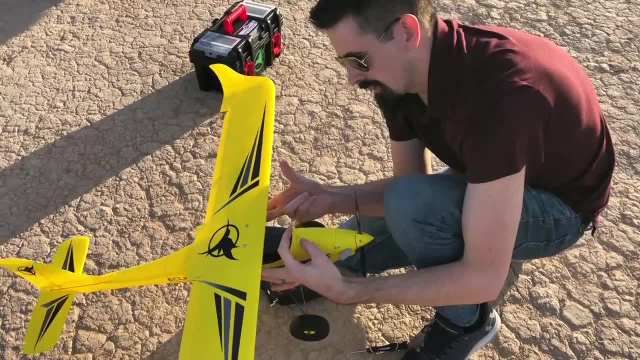 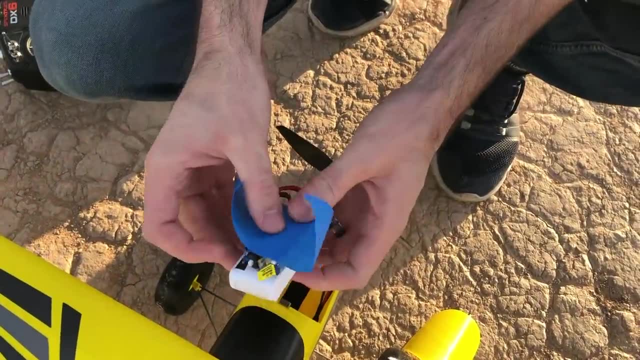 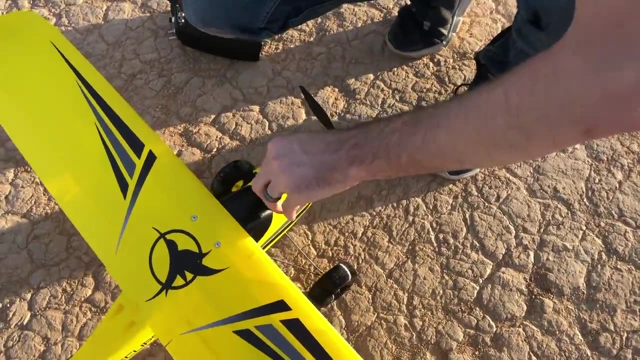 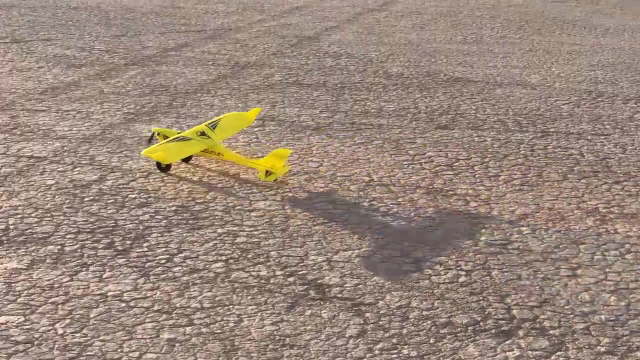 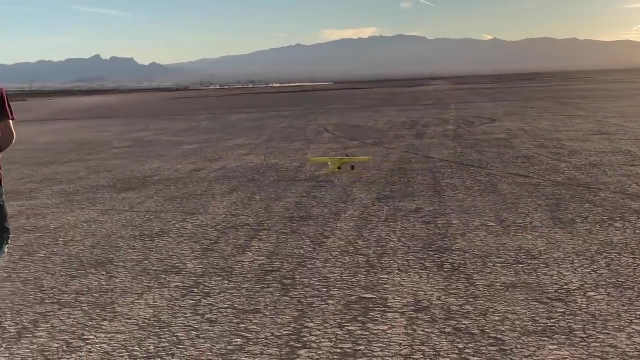 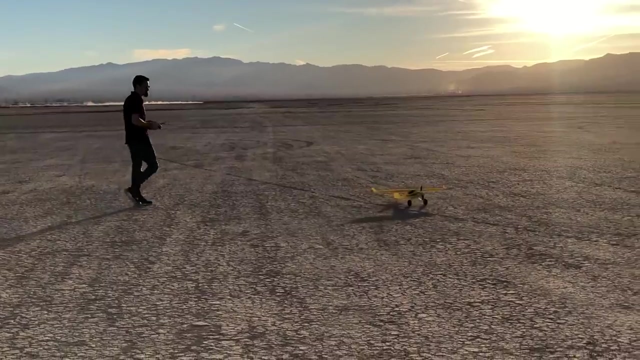 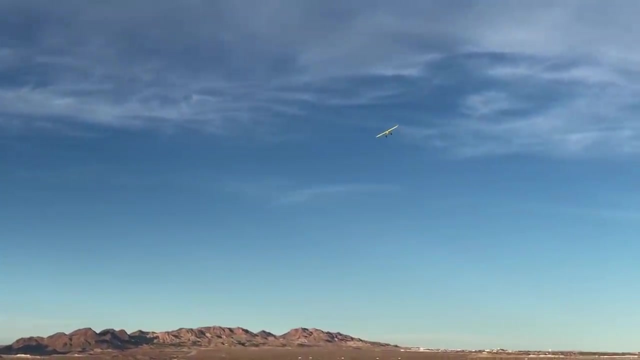 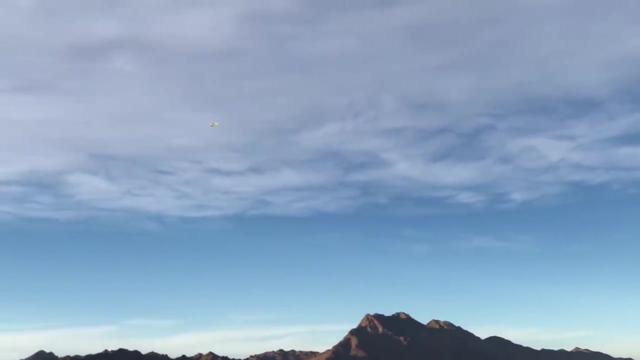 Compared to the lightweight PLA version. so I might have to add just a little bit of weight in that nose to get the To get the CG set right. Alright, so we have the PLA version up. All right, so we have the PLA version up. 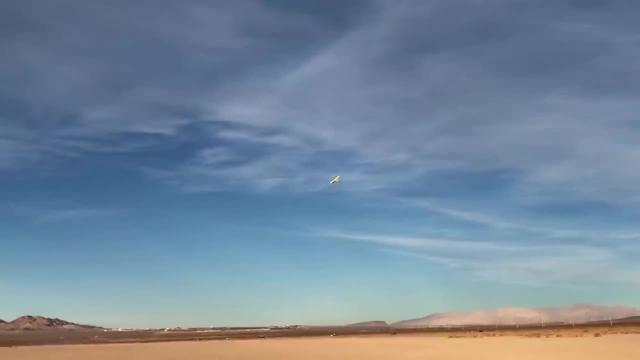 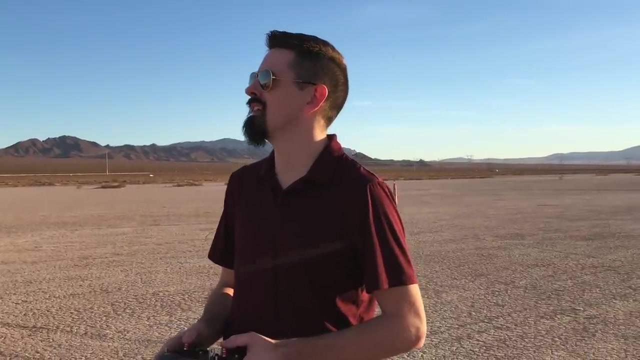 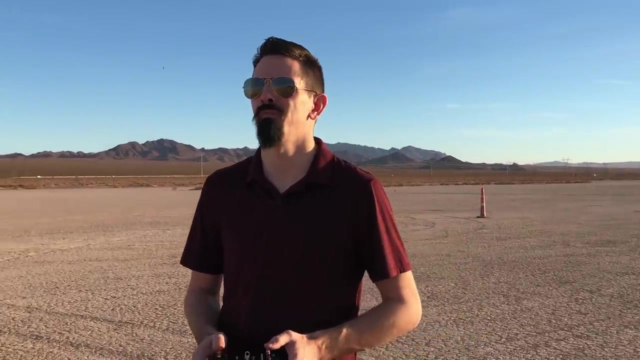 This doesn't fly nearly as good as the lightweight PLA version. It takes a lot more ground roll to get off the ground, having to have a lot more power in to keep it up in there, and Still flying okay, though, you know, and the CG was a little bit of a problem. 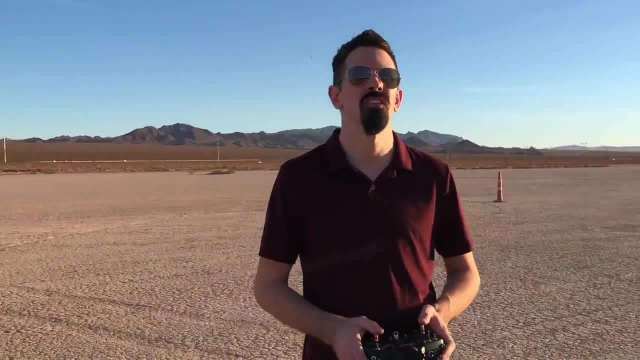 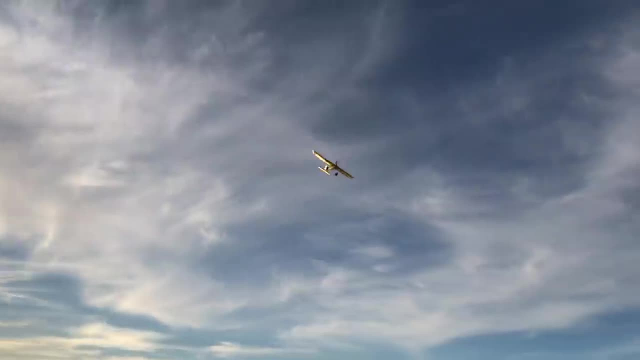 I think the CG is still a little bit aft, so I'm just being kind of cautious with it. Don't want to stall it really, Because I think it's a little tail heavy And I know it'll be pretty tough for these guys because it's a Neredle-esque thing. 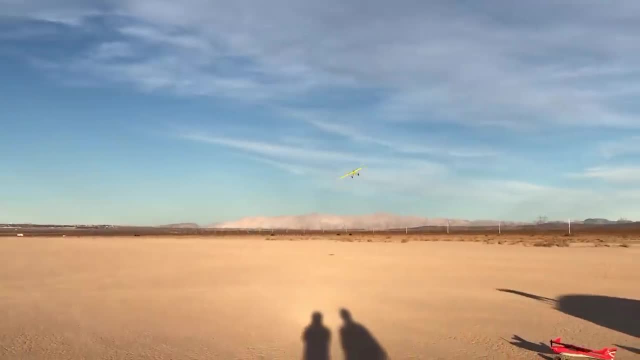 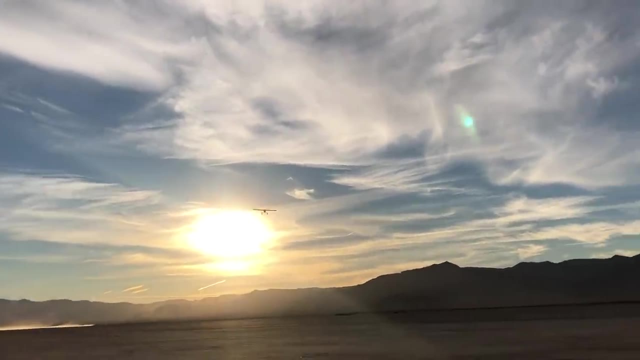 But I'm trying to get it right- The fact that you can get a better grip on the model. I think that's pretty cool. I think it'd be good if they added- or maybe they didn't, because I've been doing things like this for almost three years- 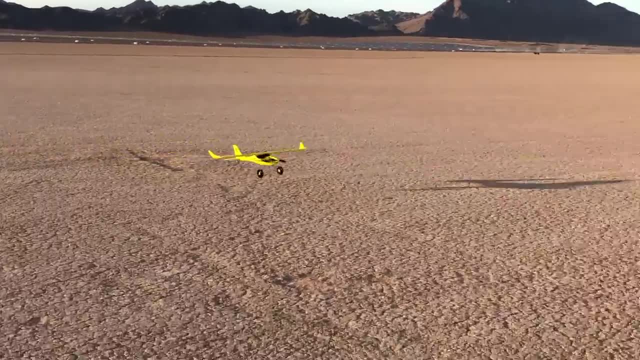 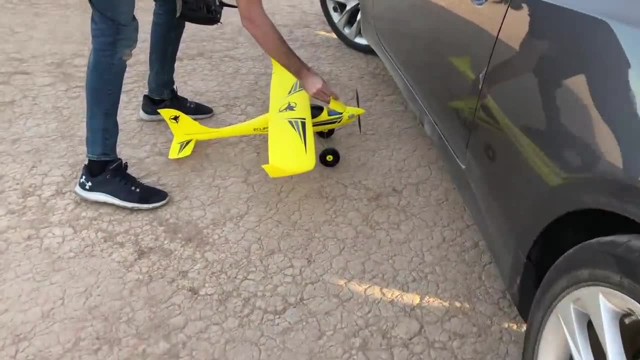 So Let's go. We've got a little bit more work to do, So let's get the pilot's done. Let's give it a second look, Some of the pilot's on a tilt, Let's see if we can get it done. All right, so first we're going to go back up to the plane. 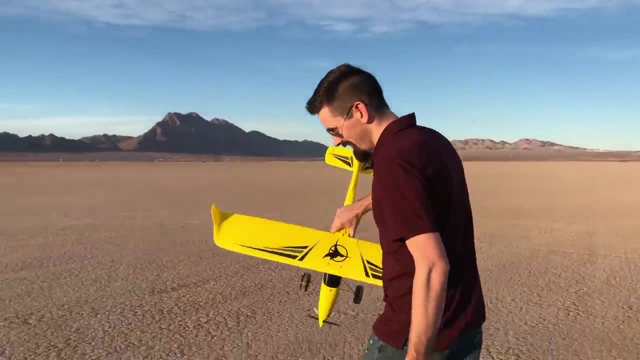 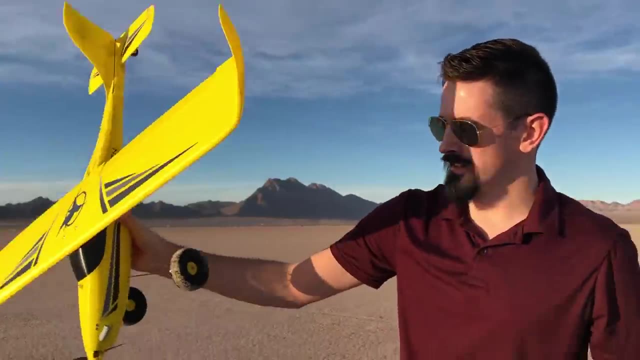 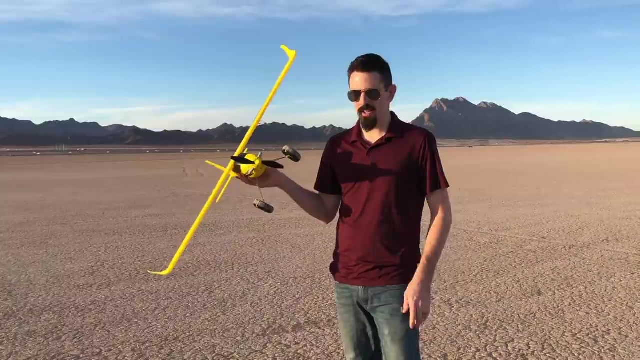 All right guys. this is a little bit of a crazy landing on that one, but it worked okay. So the sense with the lightweight or the PLA version is, you know, definitely was a handful to keep in the air. The biggest problem, I think, was the motor setup I have for it. 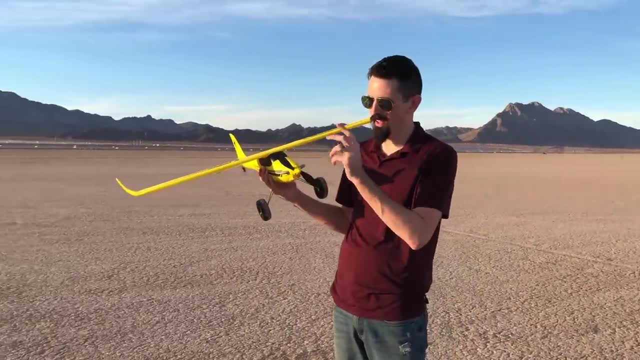 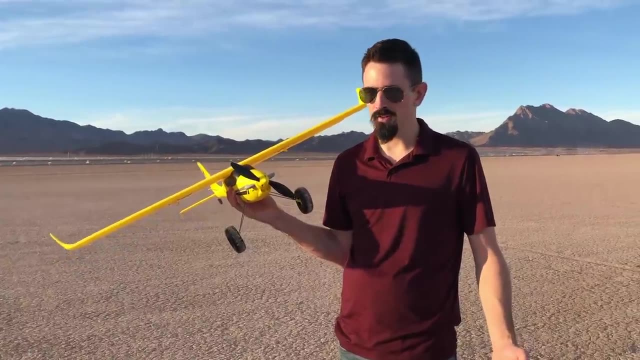 I have a 980KV motor in here and that's what I have in the lightweight PLA version and it works really really well for that, just because I'm trying to go for that slower flight kind of characteristic. So definitely for this airplane, it's way faster. 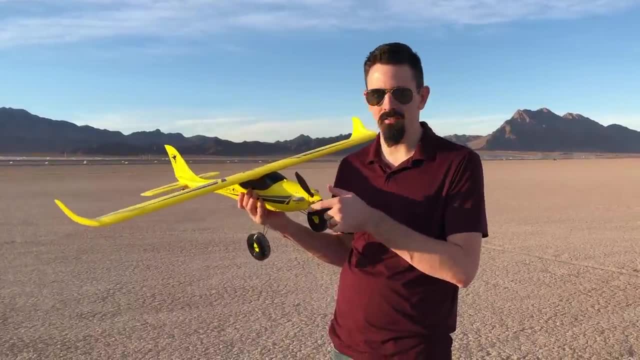 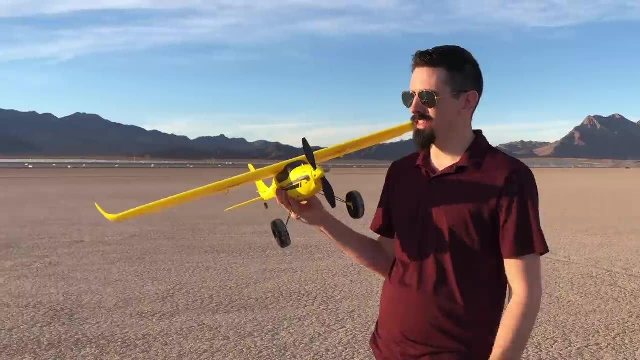 You have to keep this plane flying faster, so it needs like a higher KV motor in it. It needs like maybe a 1,400KV motor and not like a slow flight prop on here. Then you could fly this thing faster and it would be better. but it's way heavier. 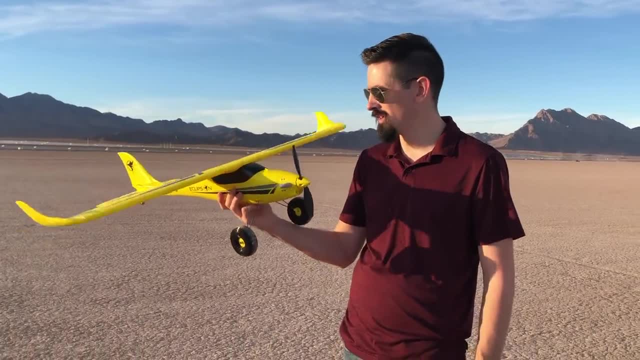 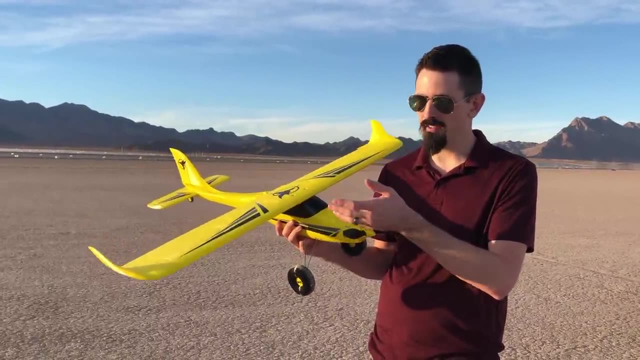 I mean you can just tell, like, how much heavier this plane is than the lightweight PLA airplane And the CG was a problem getting that set, so I had to add quite a bit of weight in the front and I already have a pretty big battery in here. anyways, as it is, 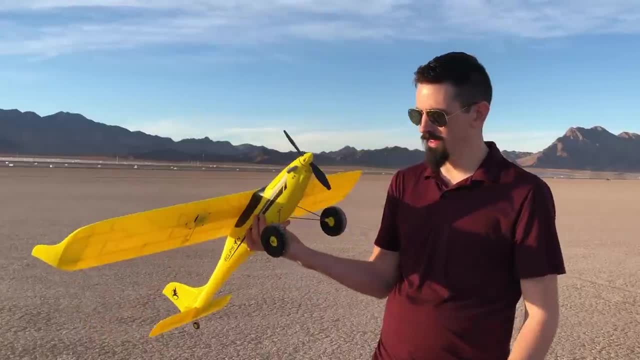 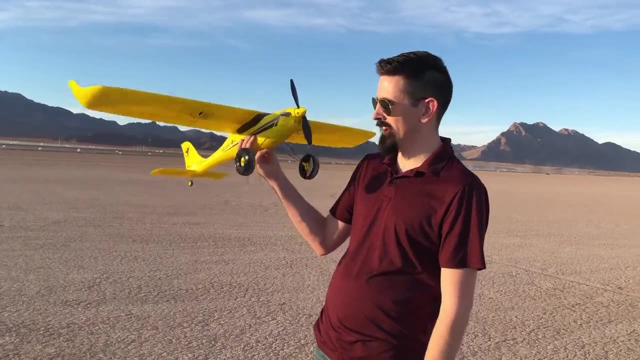 So that was a problem getting the CG set. So definitely, having like an AF-CG kind of underpowered, it just flew really hard And, like I got in a couple situations where I almost stalled, it, almost crashed it. 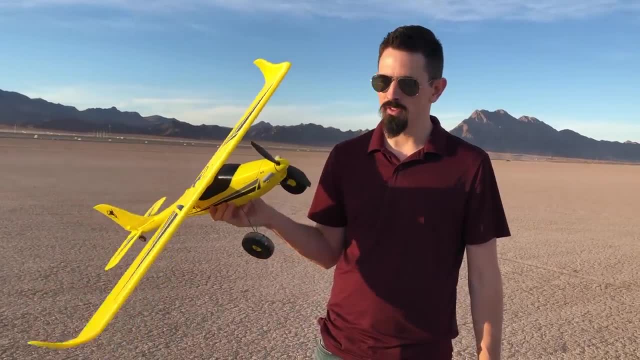 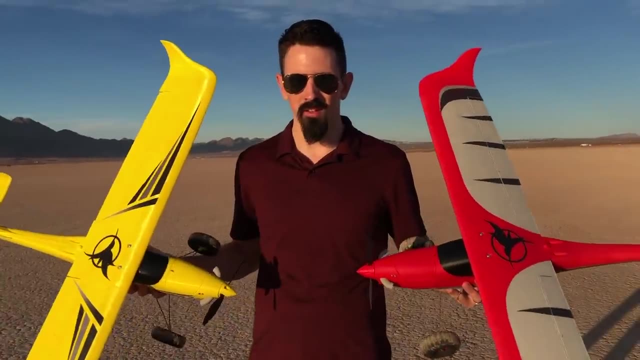 and the landing was really bad because it was just wasn't really controlled. So okay, you guys, to sum up this video, if you guys can print out a lightweight PLA, I definitely recommend it. It flew way better than the PLA version.